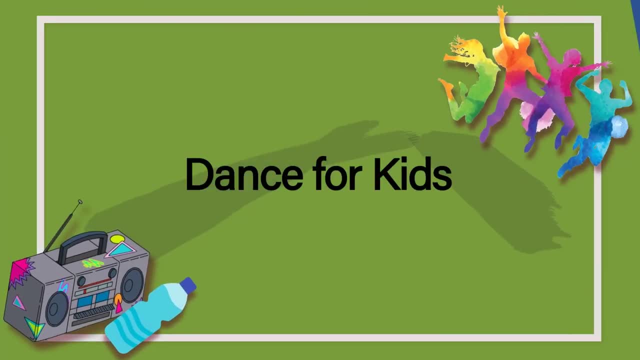 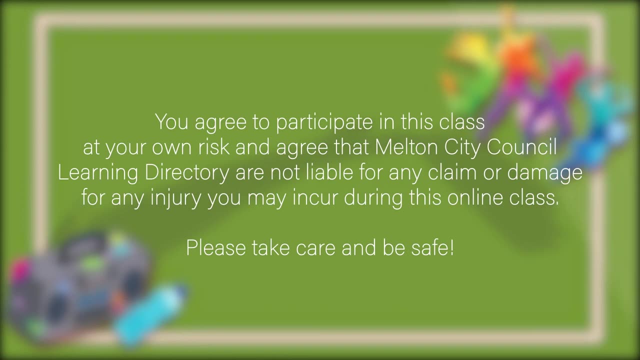 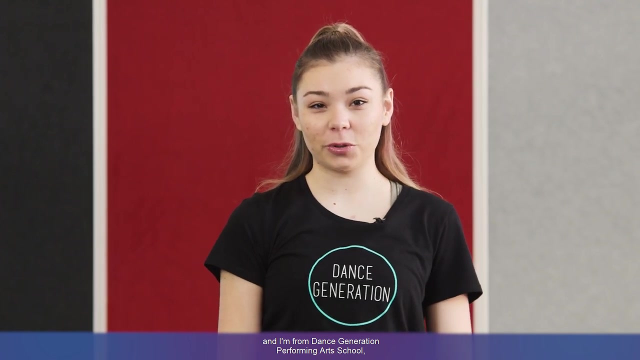 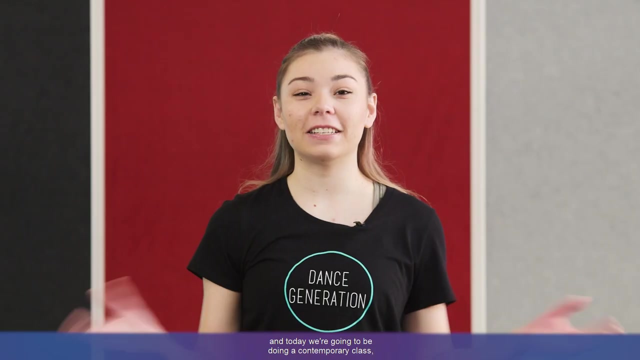 Hi everyone. I'm Ebony and I'm from Dance Generation Performing Arts School and today I'm here at the Melton City Council Learning Directory and today we're going to be doing a contemporary class. So this is for the ages of five to eight. It's a little bit challenging. 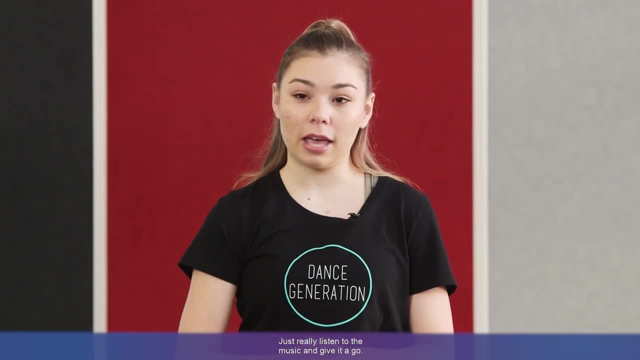 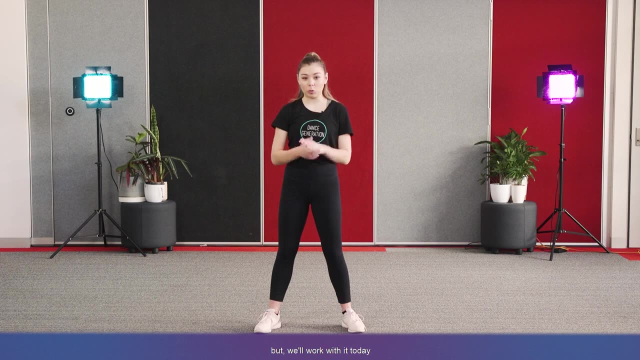 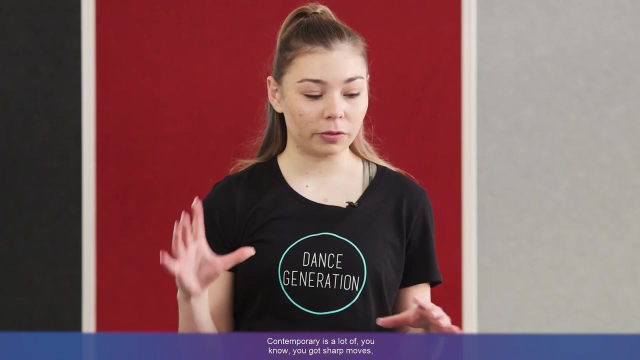 lots of fun, though. Just really listen to the music and give it a go. This is one of my favourite songs. It's a little bit different from the original, but we'll work with it today and just have a lot of fun. Just really flow through the music. Contemporary is a lot of. 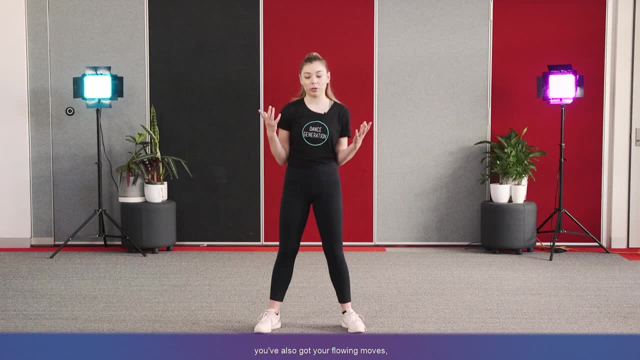 you know you've got sharp moves, you've also got your flowing moves, So just really go with it And all you have to do is feel the music and be yourself. So we're going to be doing a warm-up and a stretch, some balancing, and then we're going to go straight into the dance. 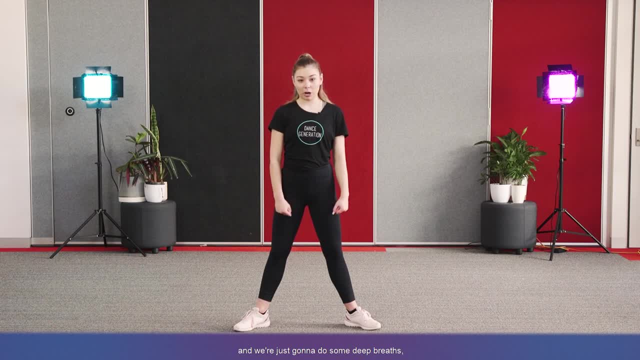 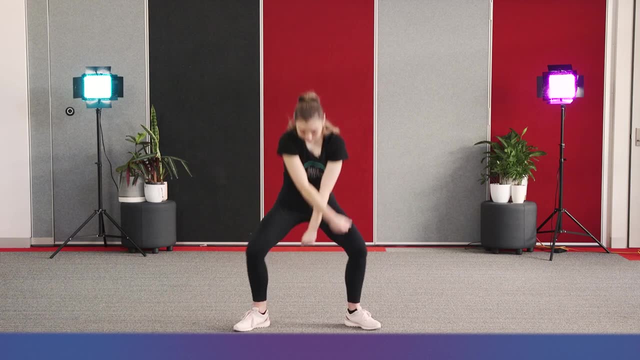 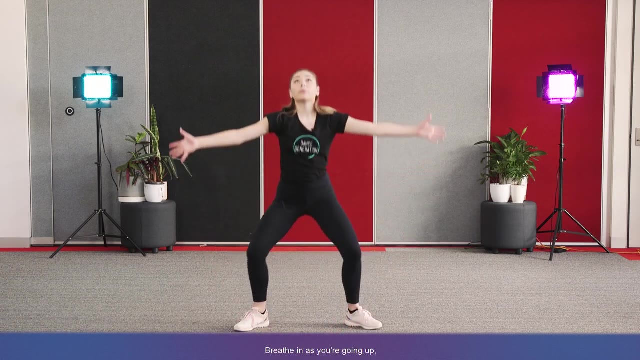 Alright, standing in second, and we're just going to do some deep breaths and we're going to do some pliés, So just follow along with me, Breathe in as you're going up and breathe out as you're going down. 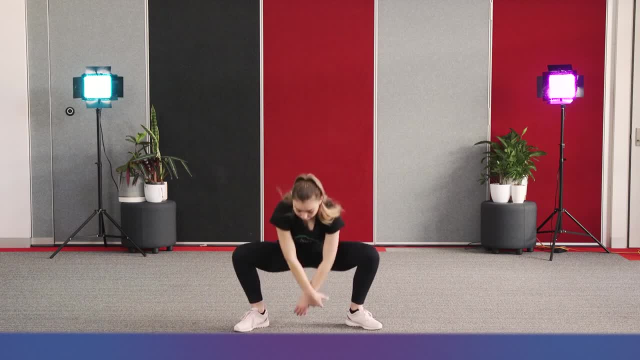 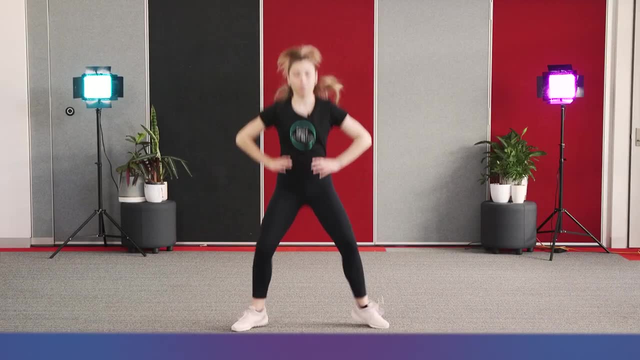 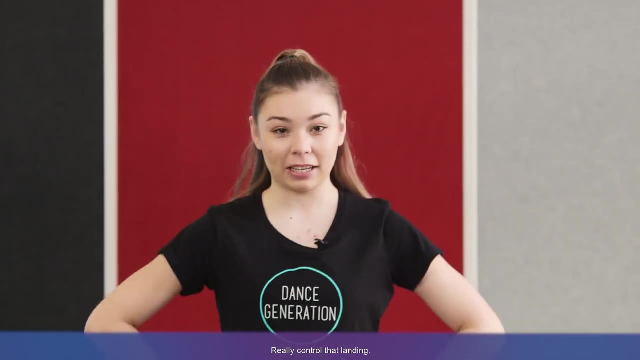 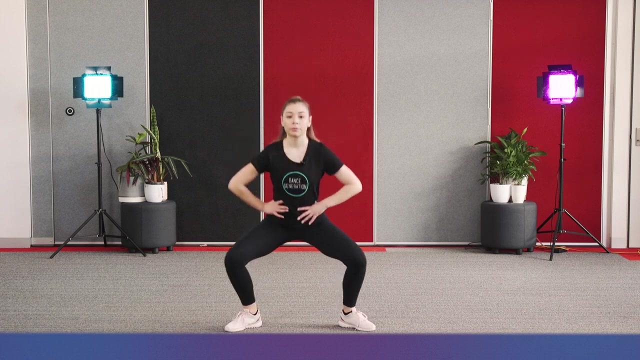 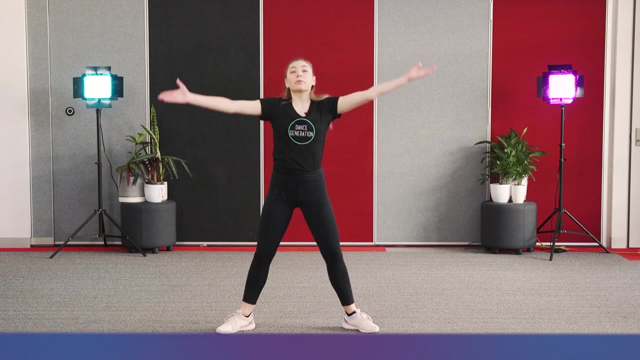 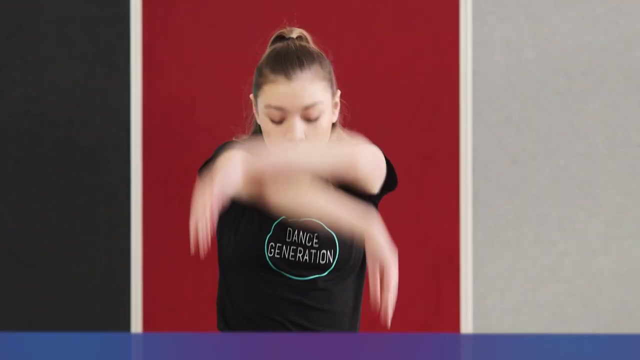 Good, Now we're going to do some pliés and jumps. Make sure to point your toes in the air. Really control that landing. Good, Beginning with our breathing. We're full. Good, Now we're going to do our jumps. 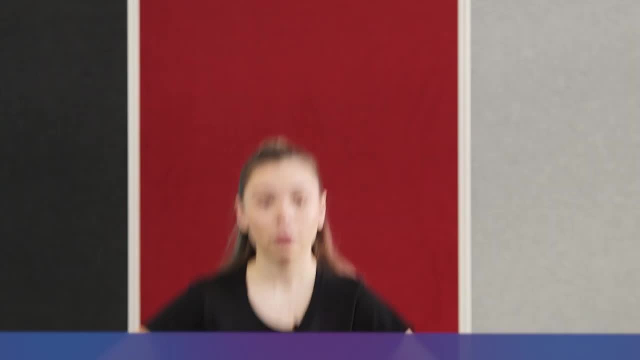 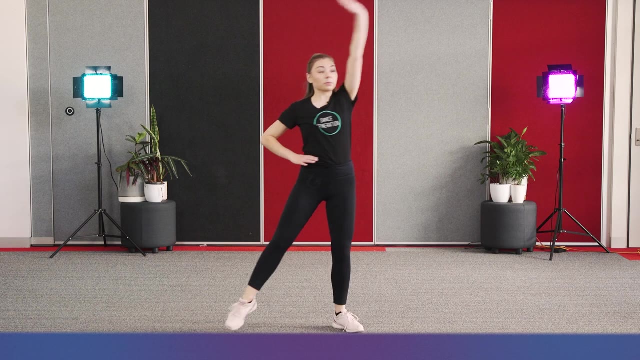 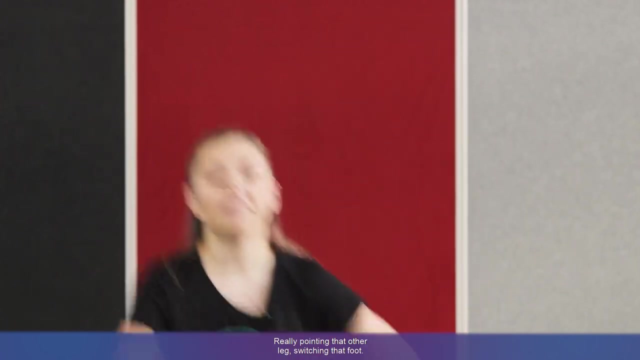 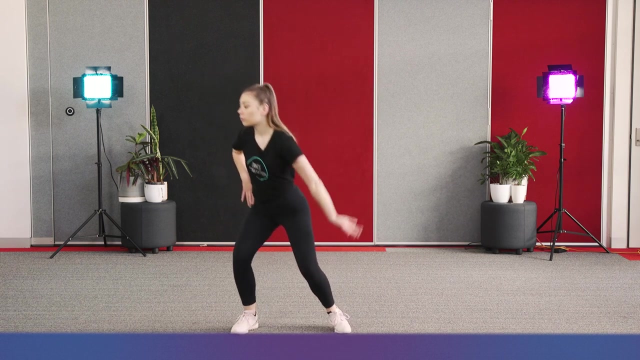 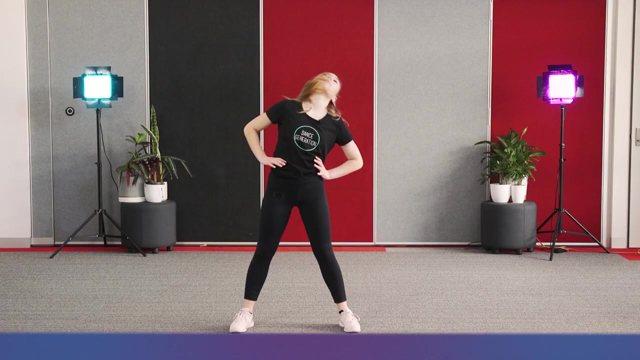 Good Streching side to side. Thank you, Thanks to ourーー. good stretching side to side, Really pointing that other leg, switching that foot. good, big rolls of the oar head, Big rolls all the way And big rolls of the shoulder. 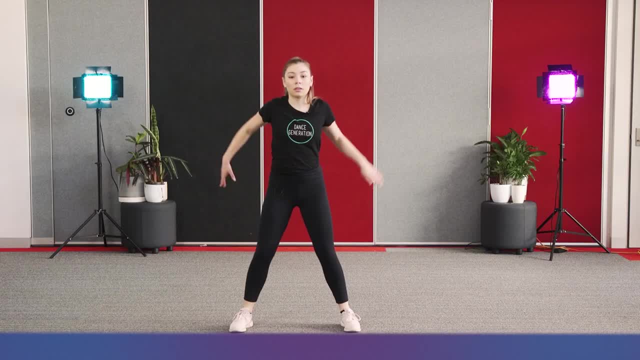 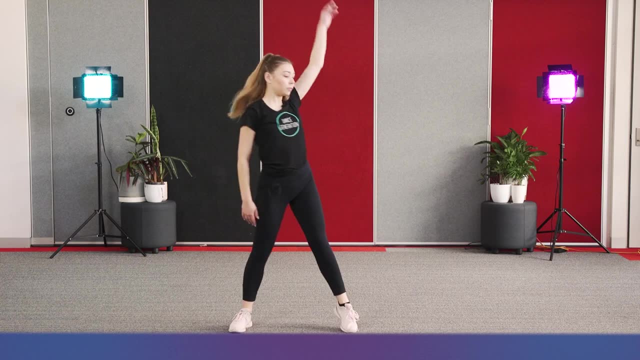 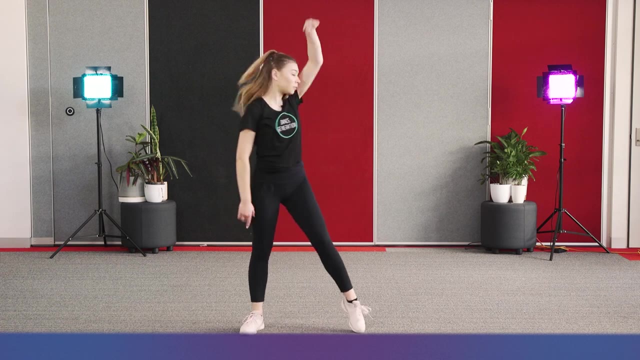 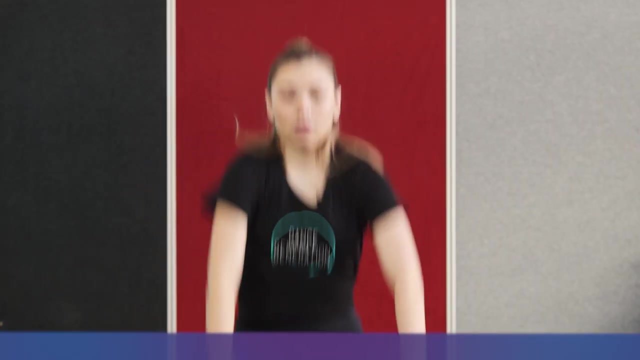 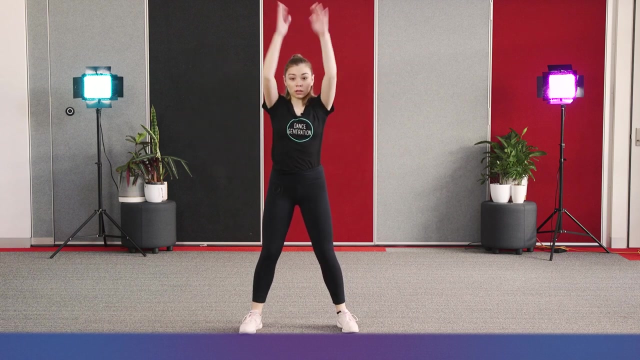 Good, Good, Good, Good, Good, Good Good. I'm running to the dawn Cause I want to live in your light. I want to live in your light, Oh, I want to live in your light In the darkest night. all I want to see is you. 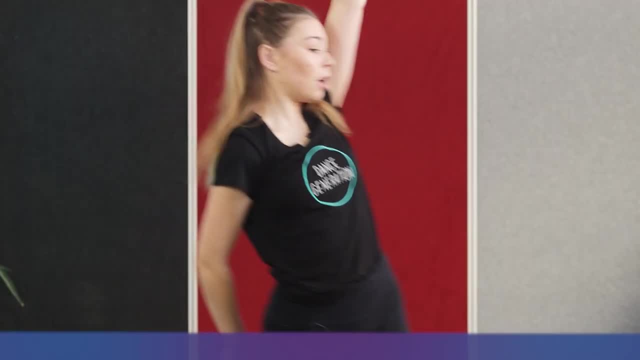 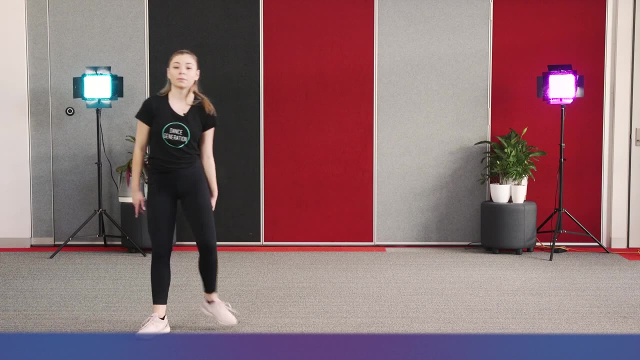 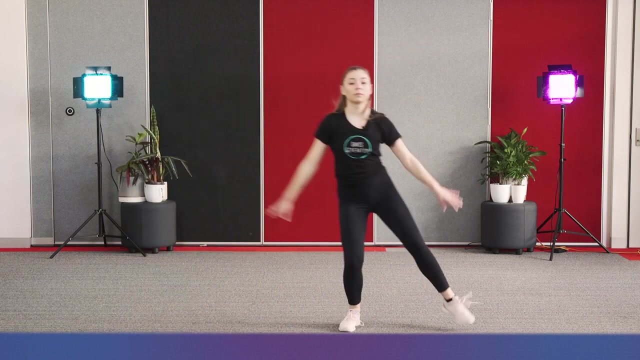 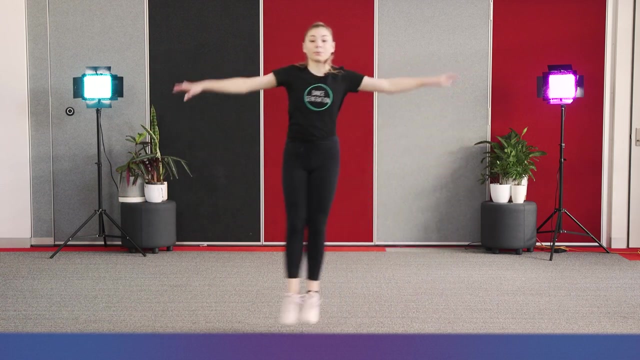 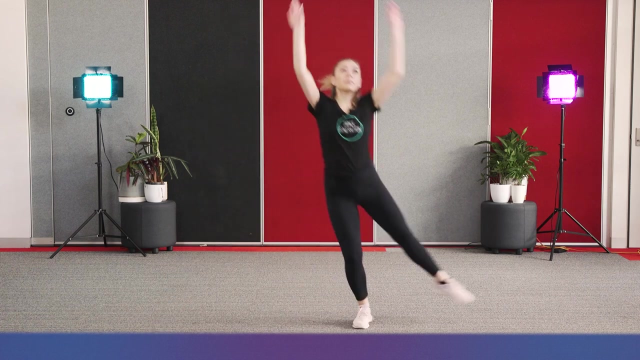 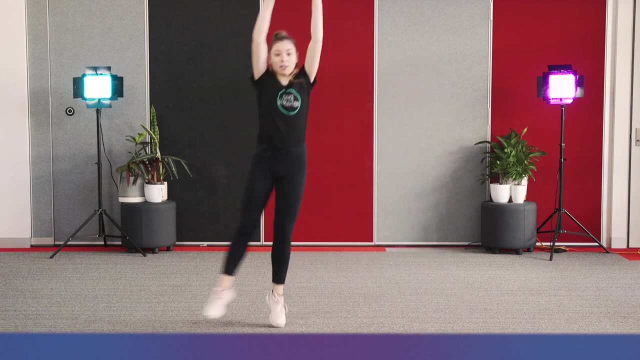 I want to live in your light. I want to live in your light In the darkest night. all I want to see is you. Oh, I want to live in your light, Cause I want to live in your light, Really pointing those toes in the air, good, and coming back to the centre- we're just going. 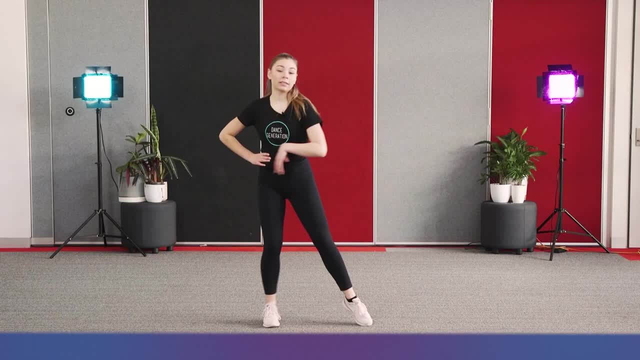 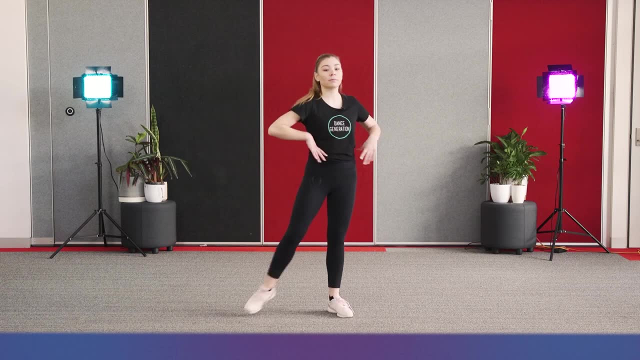 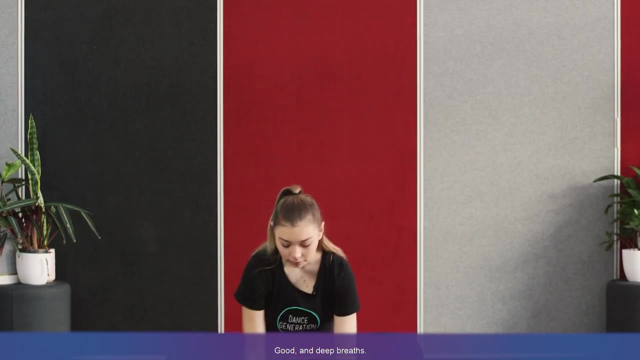 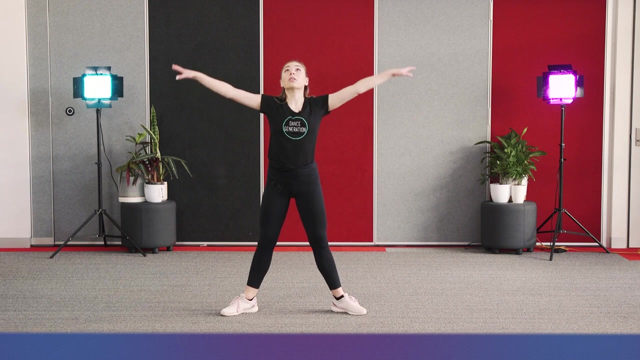 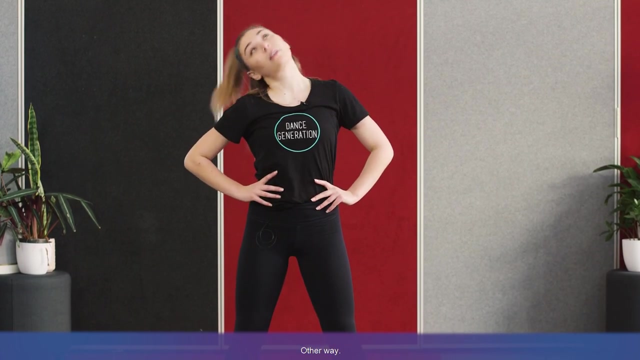 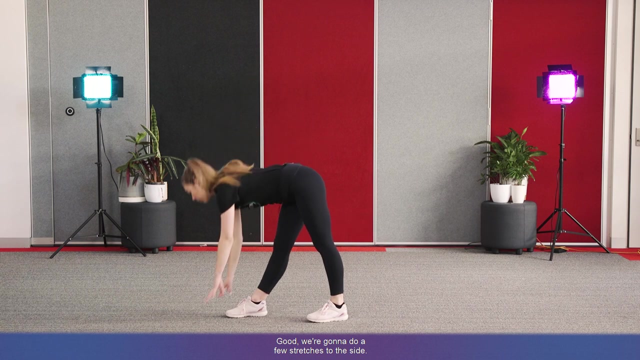 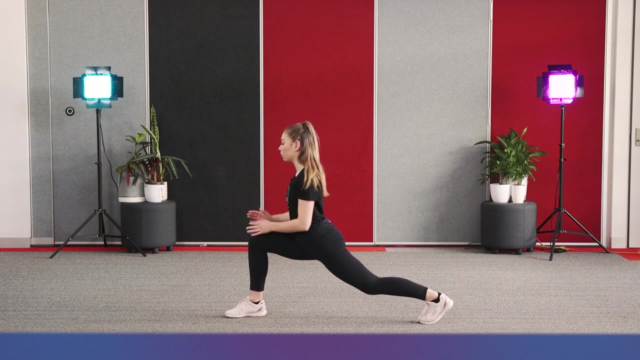 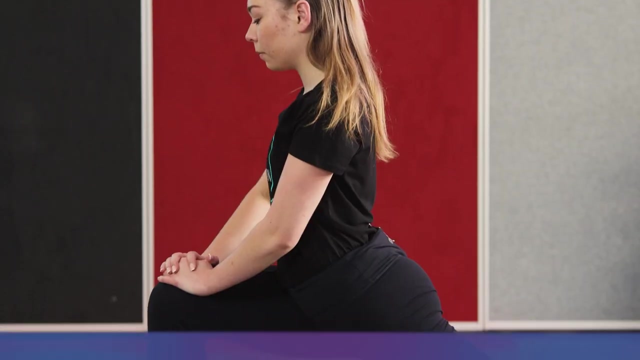 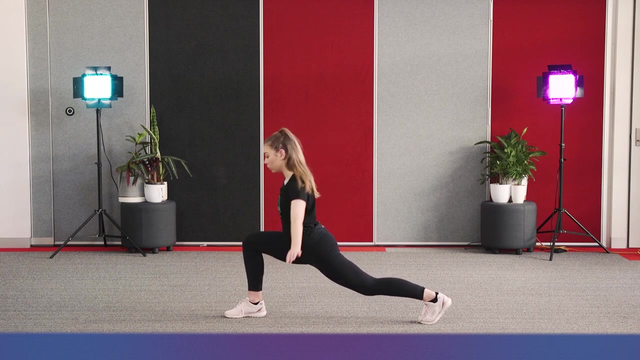 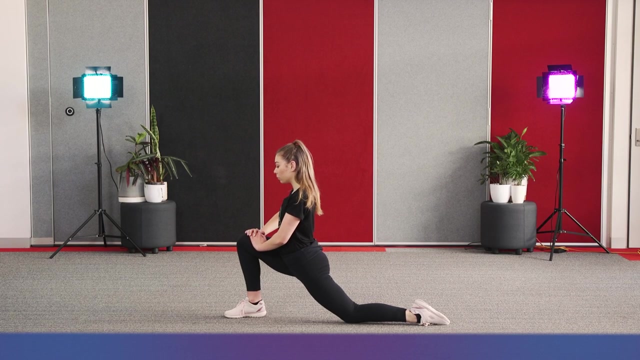 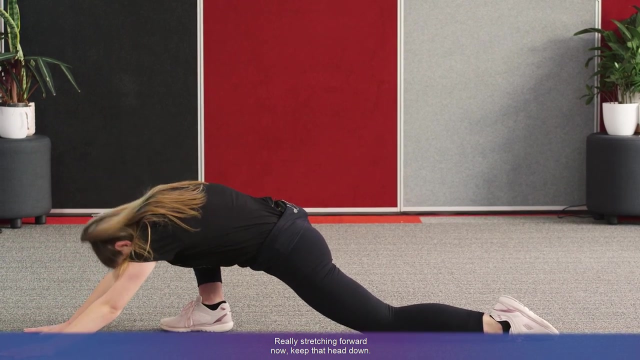 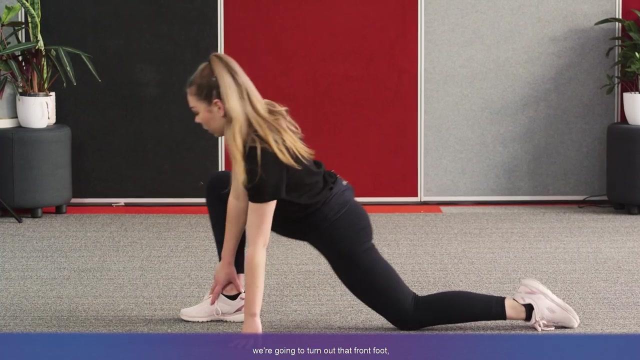 to do an easy turn and point: good, and deep breaths good, and a few head rolls again. other way: good, we're going to do a few stretches to the side, Really stretching forward now. keep that head down Now coming back, we're going to turn out that front foot and we're going to get our elbows to the ground. 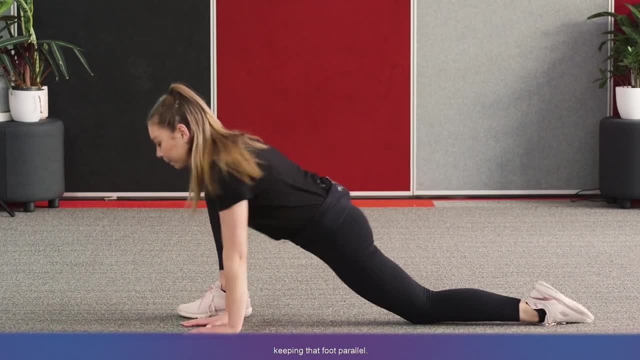 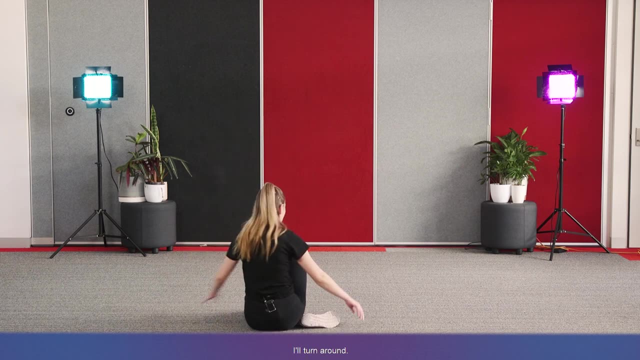 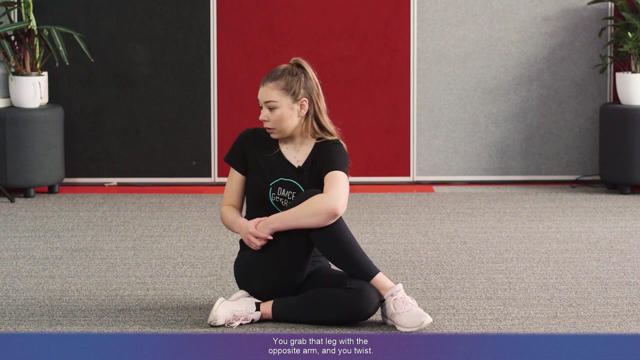 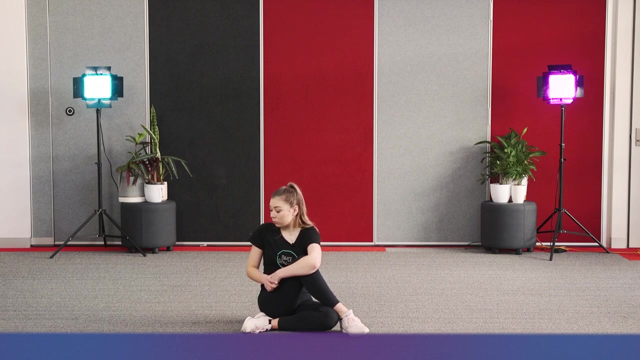 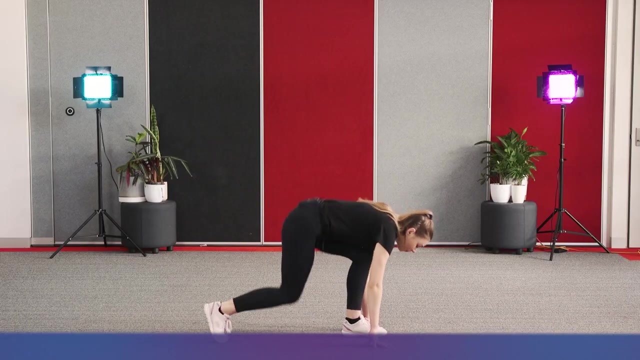 And stretching up to lizard position again, keeping that foot parallel. From here we twist and we grab That knee. I'll turn around. You grab that leg with your opposite arm and you twist. Good work, other side: Music playing. Music playing, Music playing. 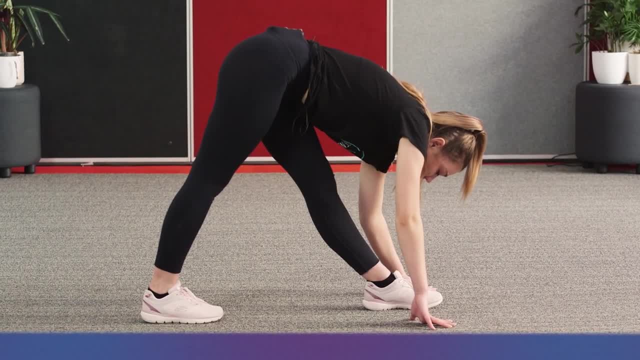 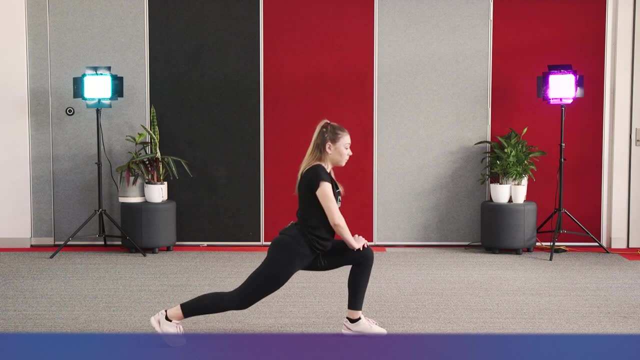 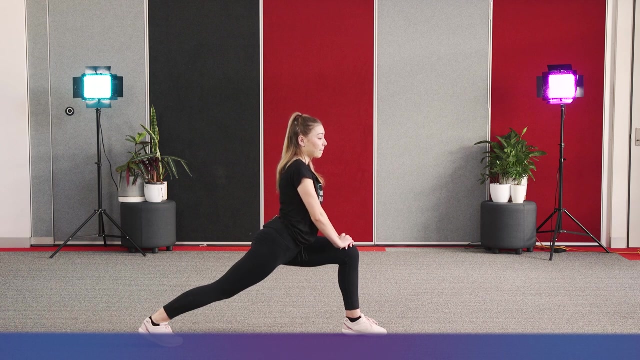 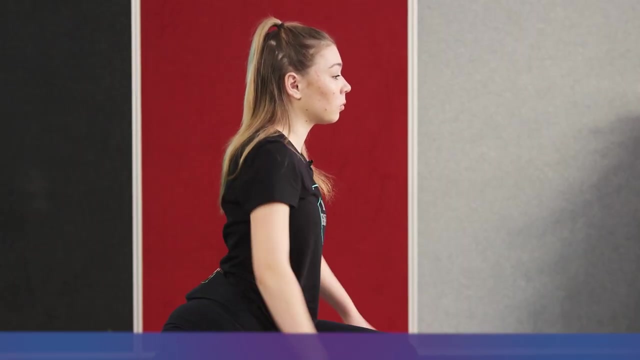 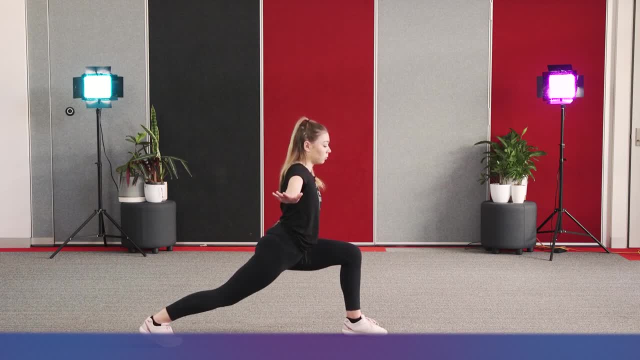 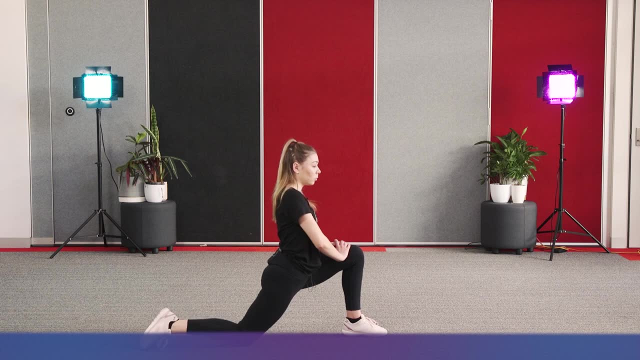 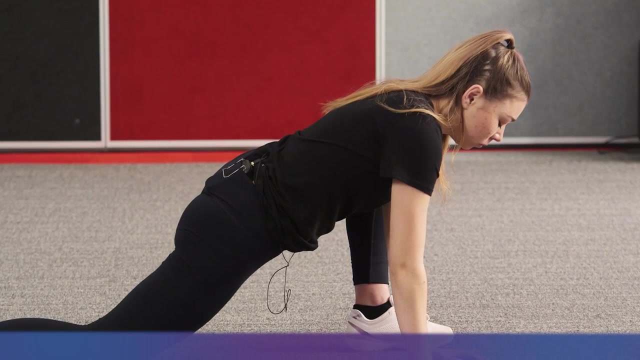 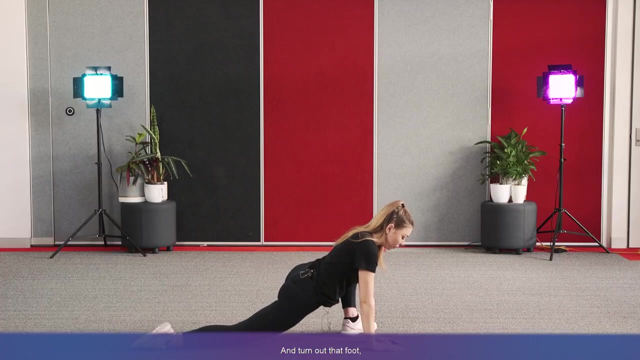 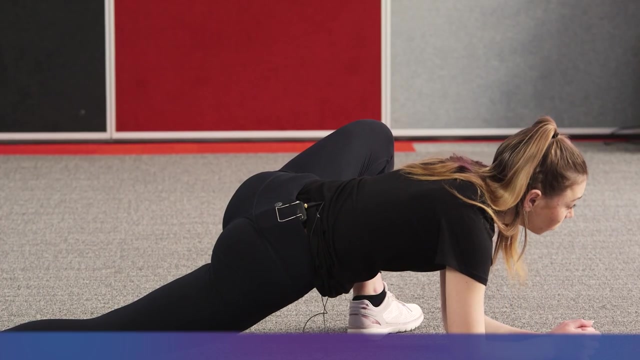 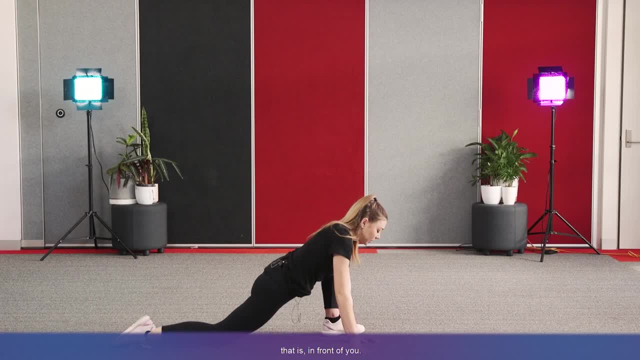 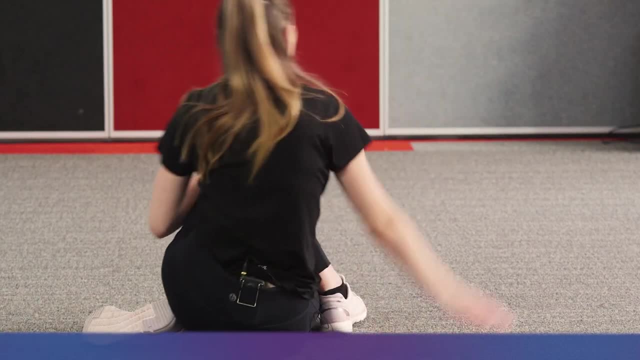 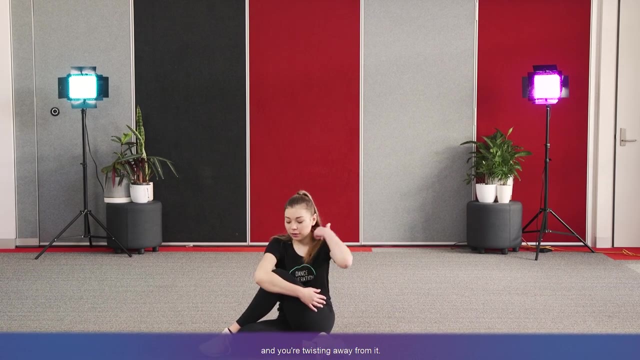 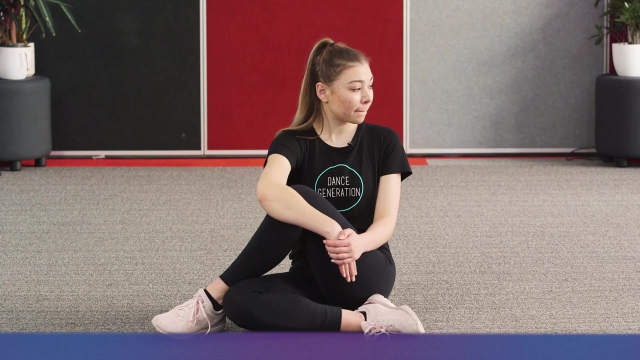 And lizard position, keeping that foot parallel. that is in front of you. Now we're going to twist to the back and I'll turn around so we can see this position. So opposite, arm to leg, and you're twisting away from it, Sitting up nice and tall. 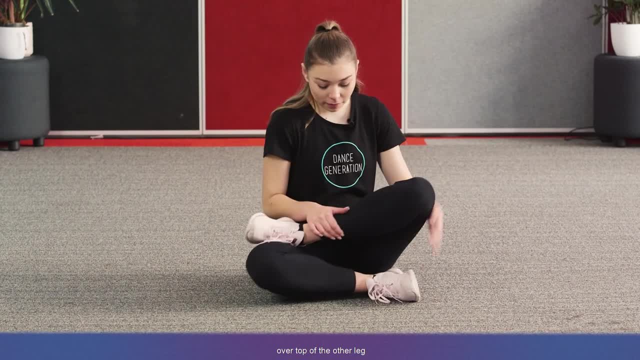 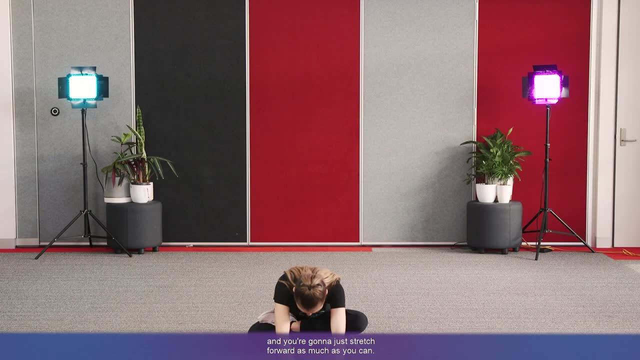 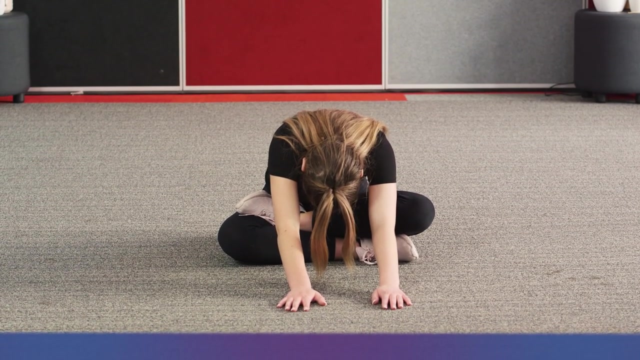 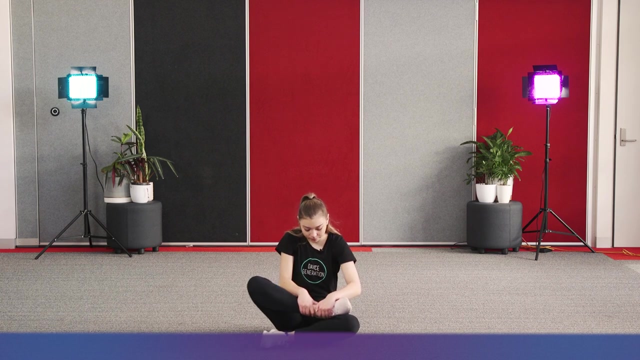 From here, you're going to put this leg over the top of the other foot, Your leg, so your feet line up with your knees, and you're going to just stretch forward as much as you can. Good, let's swap legs And reaching forward as much as you can. 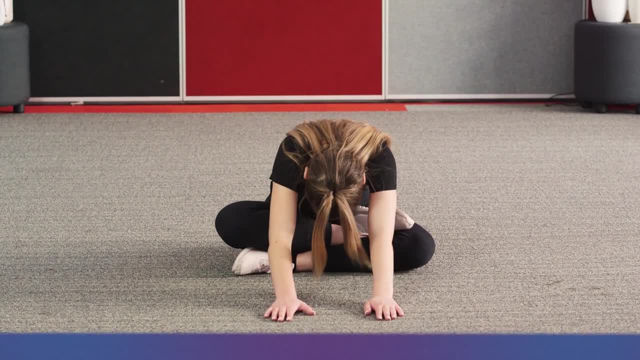 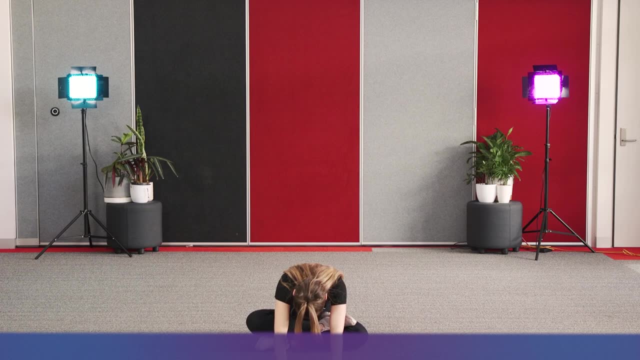 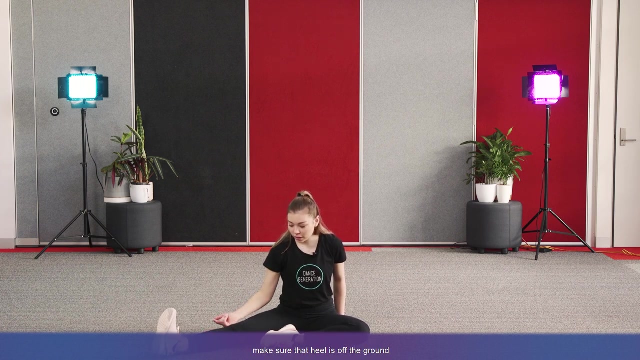 Good, Good, Good, Good, Good, Good, Good. From here, stretch that leg out to the side and we're going to flex it up. Make sure that heel is off the ground. if you can make it there, Then we're stretching over, so really stretching that side out. 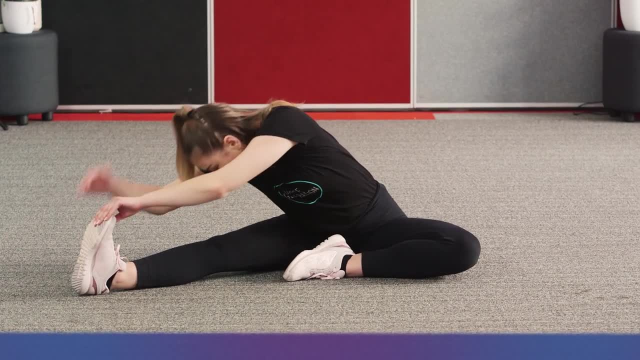 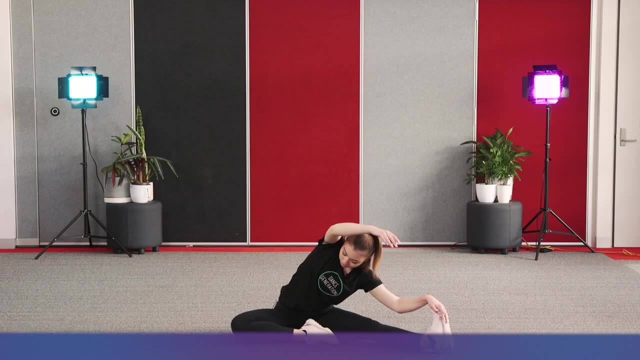 And looking down at your knee and reaching for that foot- Other side- Good, Other side- And twist, Good work. From here you're going to sit like a split-like position, Your foot is wherever it's comfortable And you're going to sit forward and you're going to sit up nice and tall. 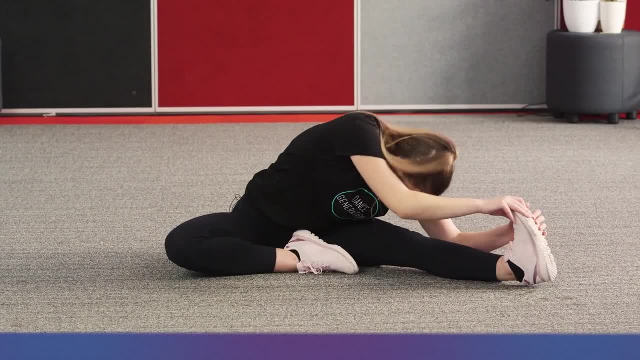 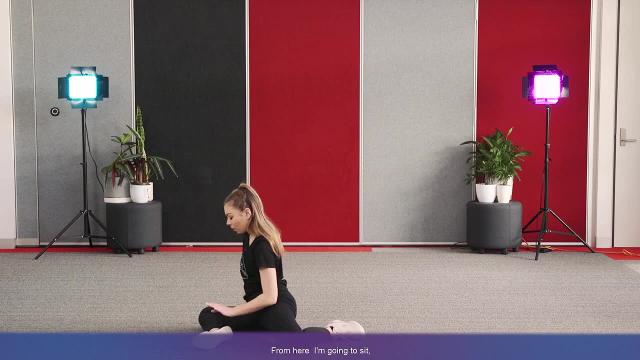 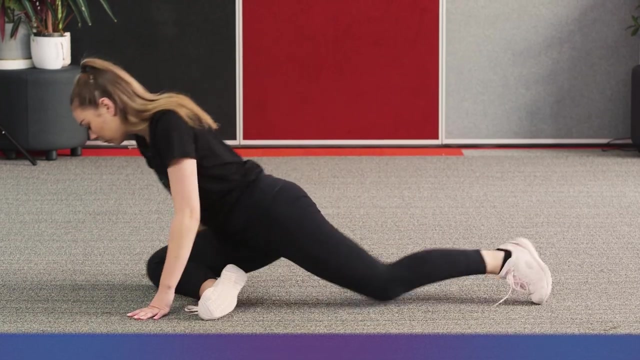 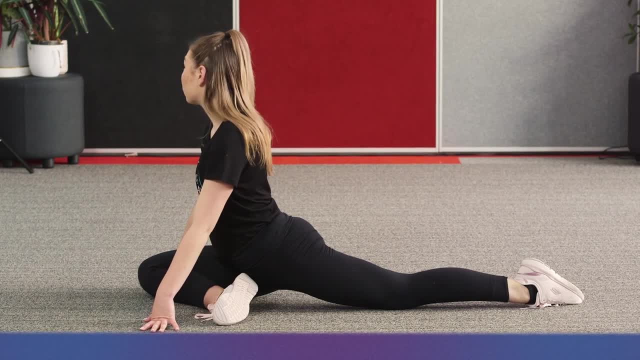 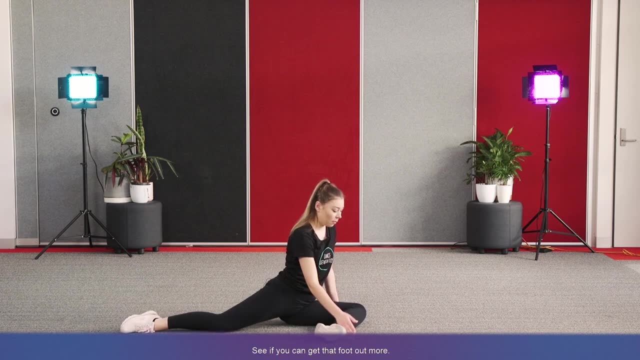 Good, Good, Good, Good, Good, Good, Good. You're starting out nice and tall. Try stretching that back leg. Good work, and try your other leg as well. See if you can get that foot out more If you can't keep it as close to you as possible so you can really stretch. 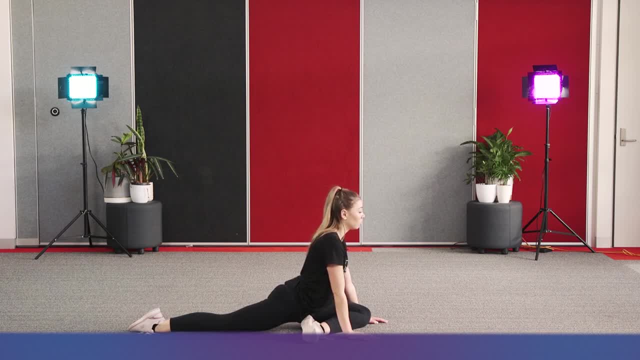 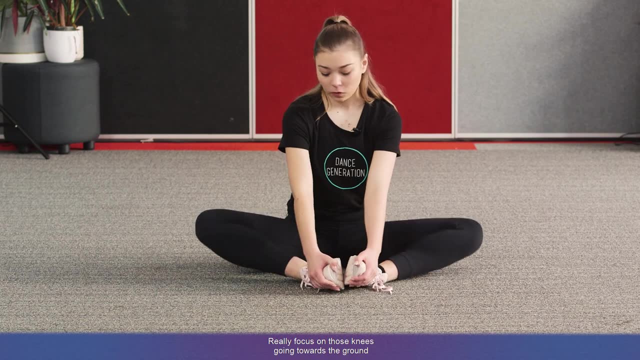 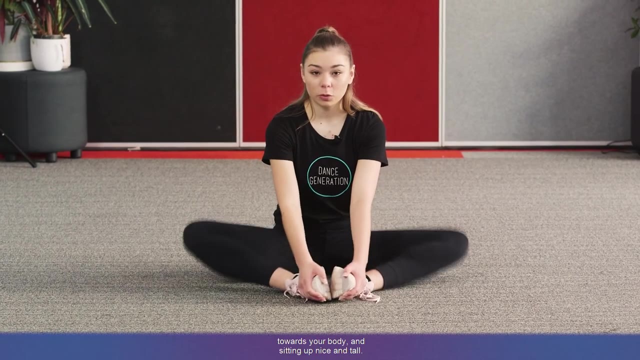 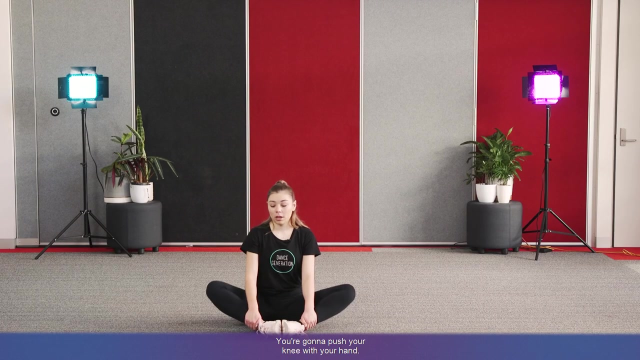 Good, and let's do our butterfly stretch: Real, simple, easy to do, Okay, Great. Really, focus on those knees going towards the ground and staying there, rather than bringing them up towards your body and sitting up nice and tall. Then you're going to push your knee with your hand- the inside of your leg, not right on. 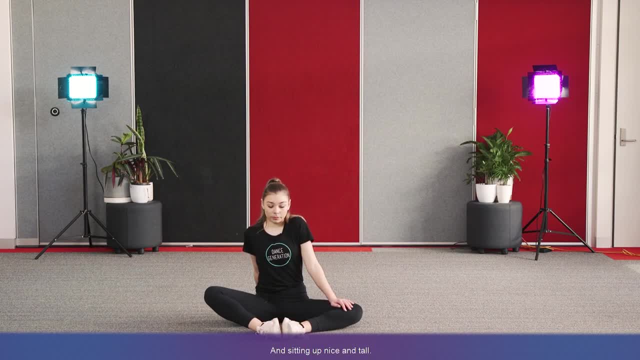 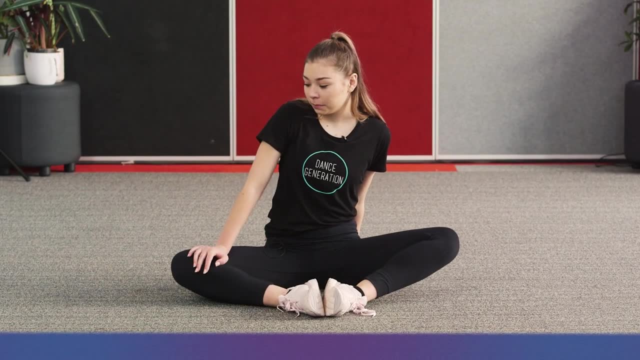 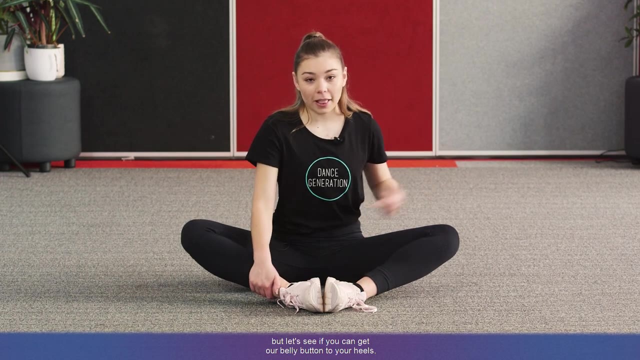 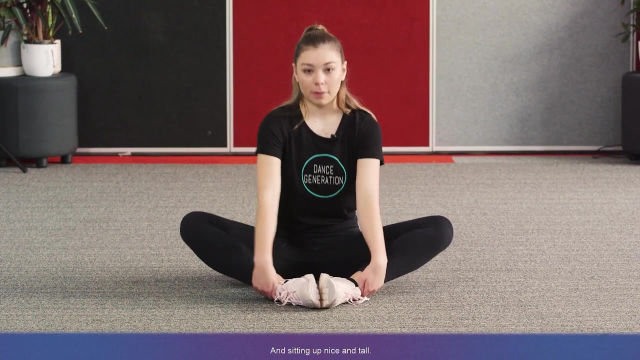 top of your knee and sitting up nice and tall. And try the other side, pushing away from that leg. And now we can all get our head to our toes, but let's see if you can get your belly button to your heels and sitting up nice and tall. 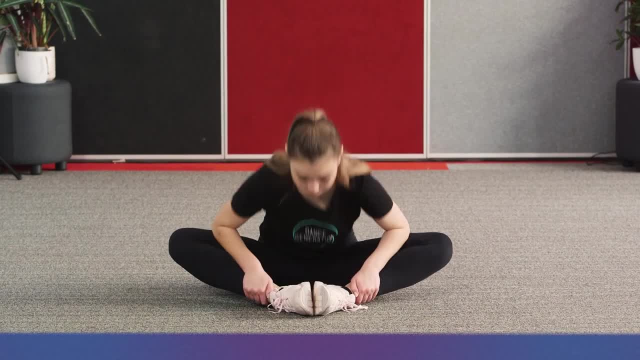 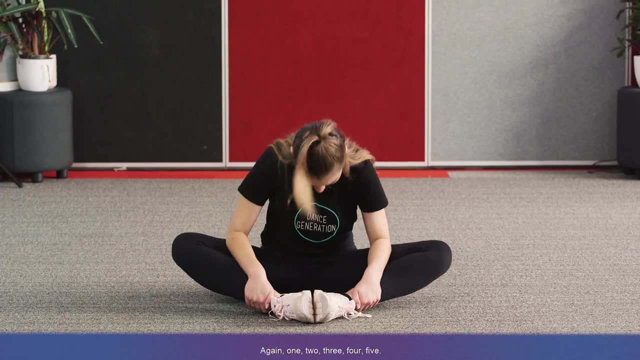 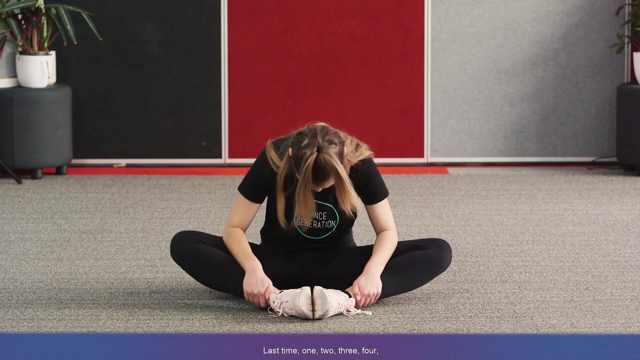 Now we're going to pulse for four and sit up on five. Let's give it a go. two, three, four, five again. one, two, three, four, five, six, four, five. last time: one, two, three, four, stretch up nice and tall. 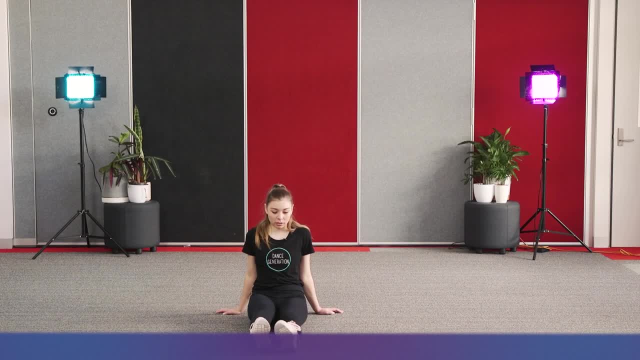 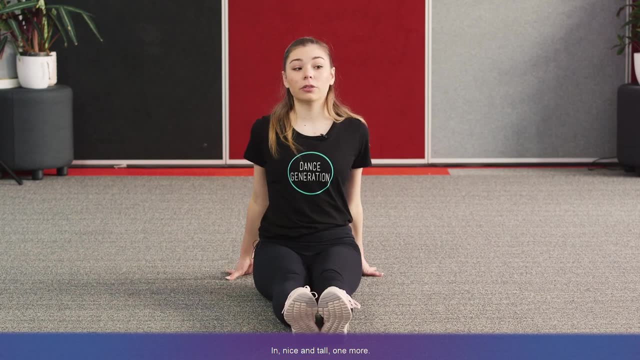 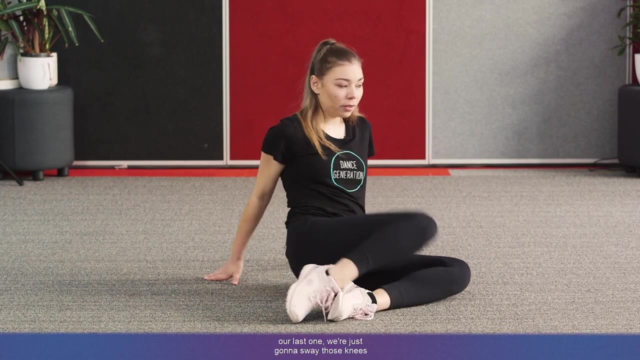 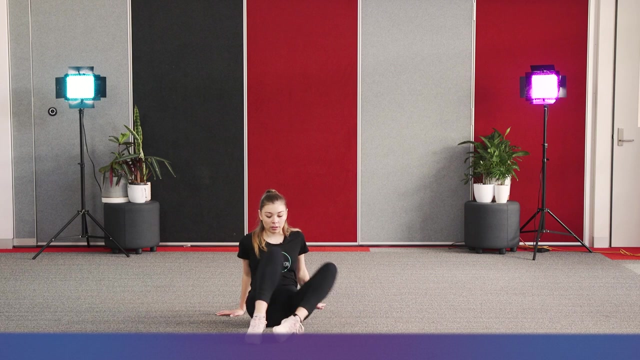 Good work. Shake out those legs. bring them both in: stretch nice and tall in nice and tall One more. really bring it in. and now our last one. we're just going to sway those knees side to side. Give me a nice toes pointed good, good job. 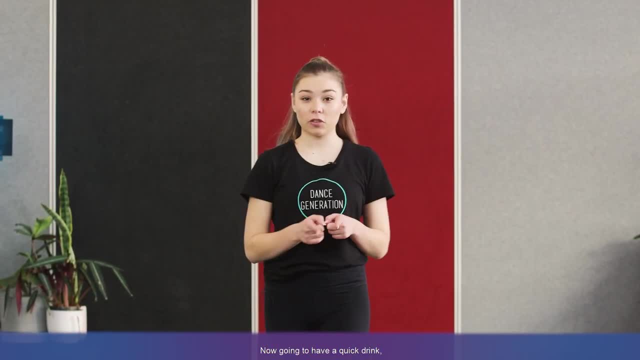 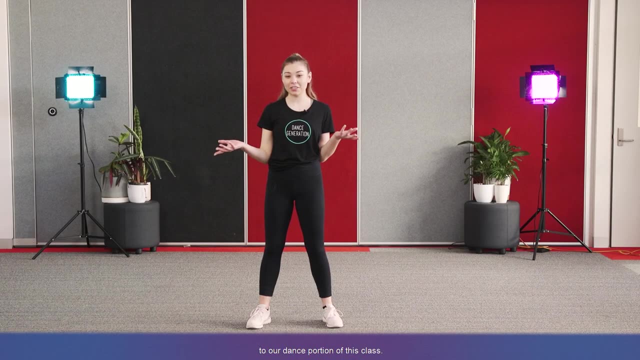 So that was our warm up and our stretch. Now we're going to have a quick drink and when I'm back we will start on to our dance. Okay, so now we're going to move on to our dance portion of this class. So today we're going to be doing the song River. 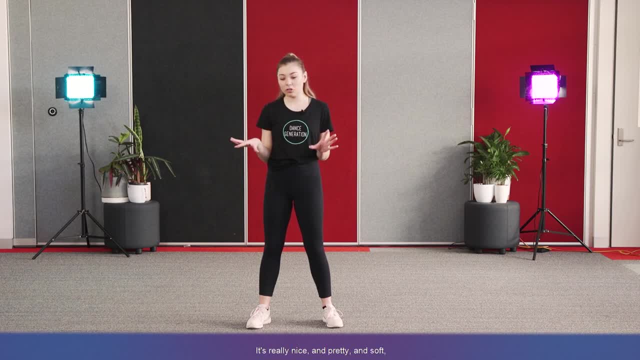 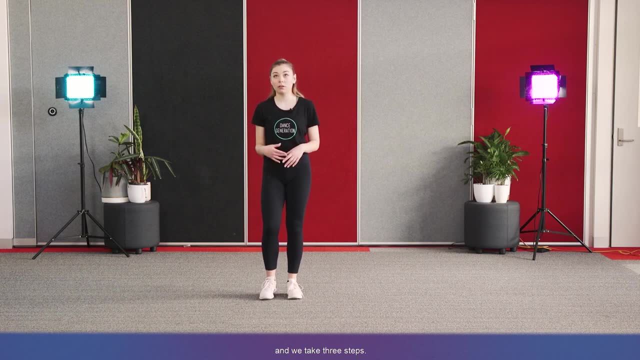 So just give it a go, really feel the music. it's really nice and pretty and soft. So just have fun. So we're going to start. We're going to start walking forward and we take three steps. our arms are just really. 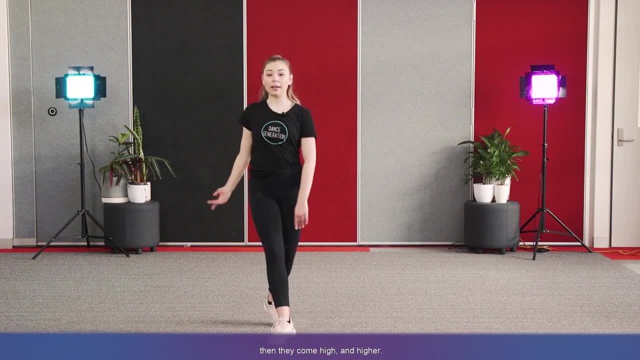 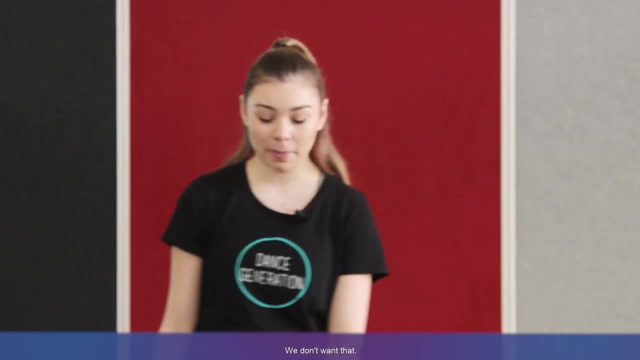 low, then they come high and higher. yes, Now I really want you to have a really tall posture, sort of being really short and slumpy. yeah, We don't want that. we want, as we step, we look up, yeah. 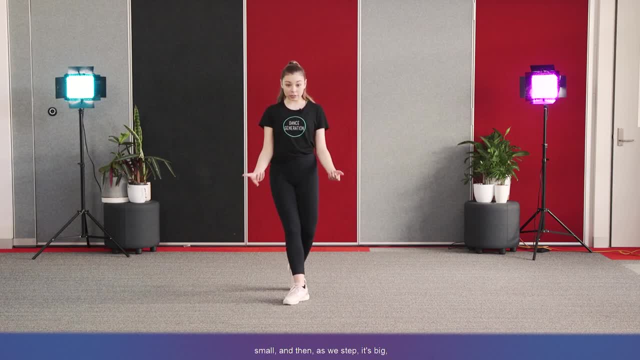 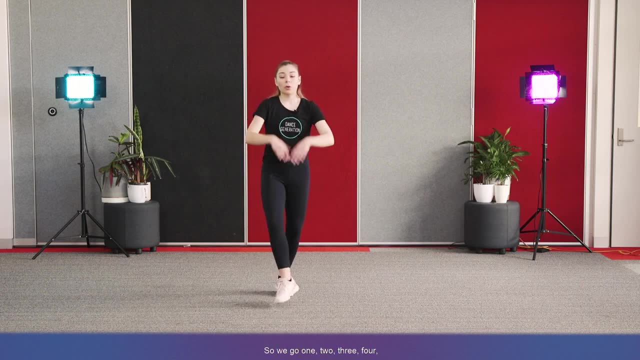 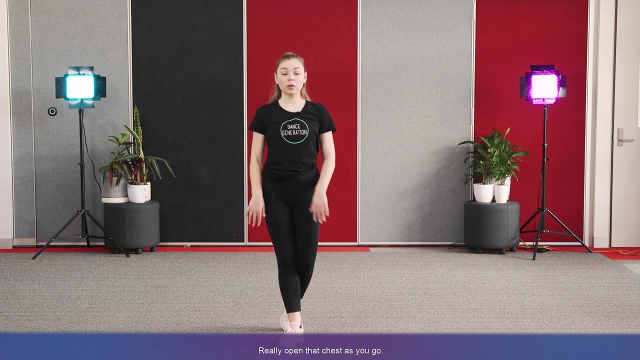 So at the start it's kind of low, small, and then as we step it's big, gets bigger each time, yep, And it's quite slow. So we go one, two, three, four, five, six, yes, 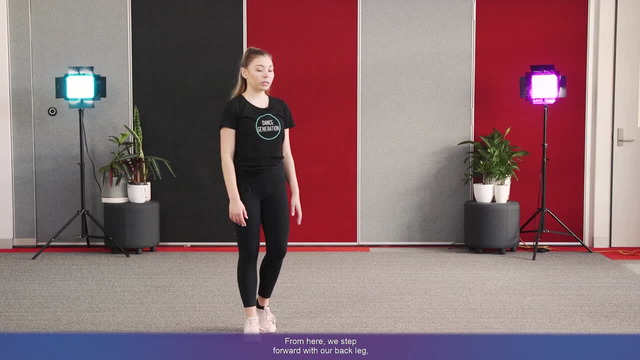 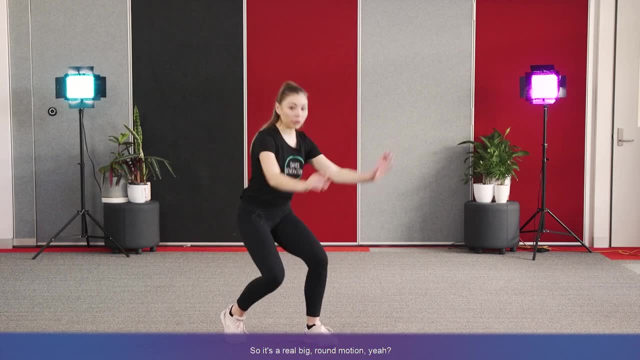 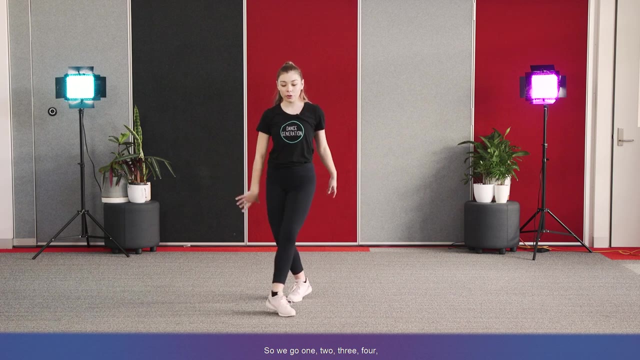 Really open that chest as you go From here, we step forward with our back leg and we push, So it's a real big round motion, yeah. So let's go from the start and we'll count it. So we go one, two, three, four, five, six. 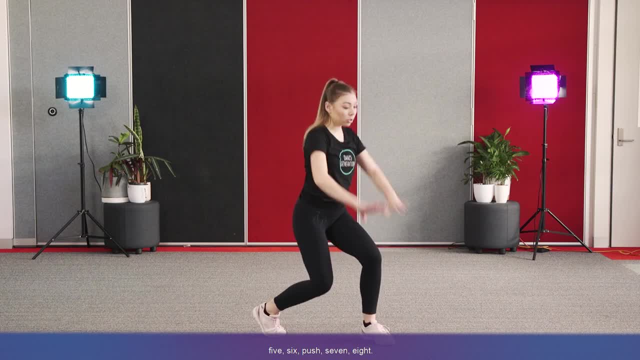 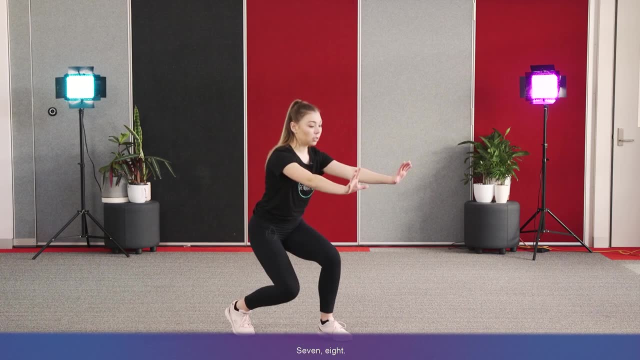 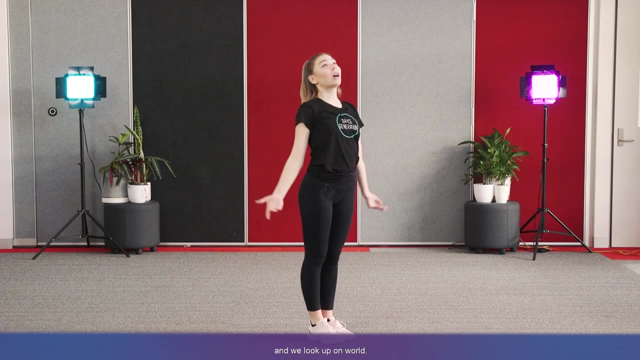 Yeah, One, two, three, four, five, six, push seven, eight. from there seven, eight, We come up and as we come up, our arms go back forward and we look up on world back open. 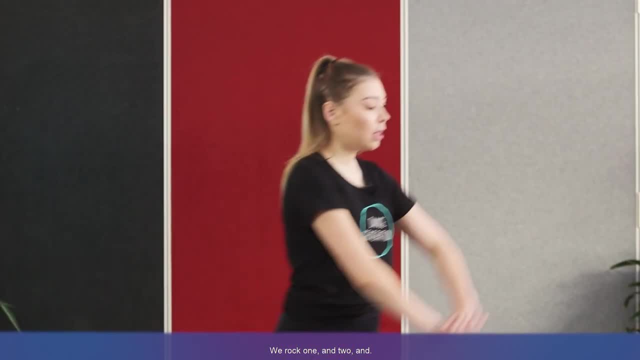 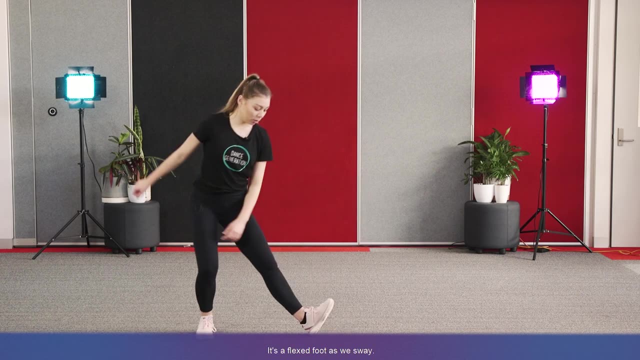 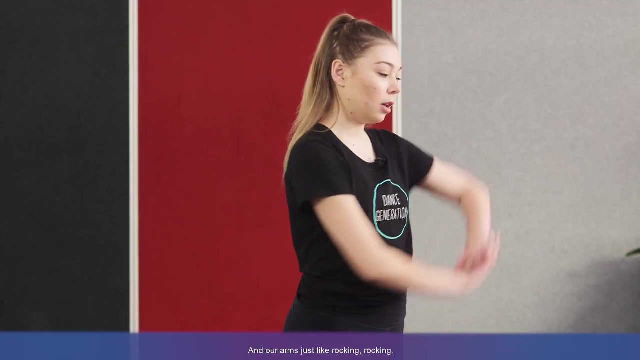 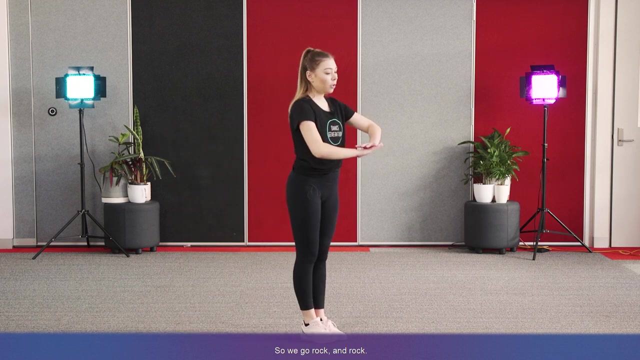 From here we rock, we rock one and two, and So just our legs. It's a flexed foot as we sway, sway up, sway together, and our arms are just like rocking, rocking. So we go, rock and rock. 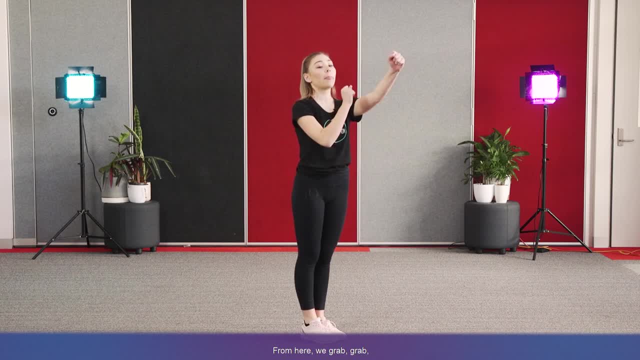 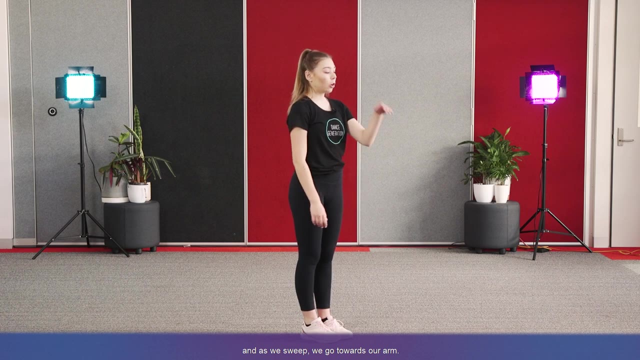 From here. we grab, grab, and then we look, we stretch, and our front leg is stretched and our back leg is bent. So we grab, grab, look, We look. From there, our arm sweeps behind us and as we sweep we go towards our arm. 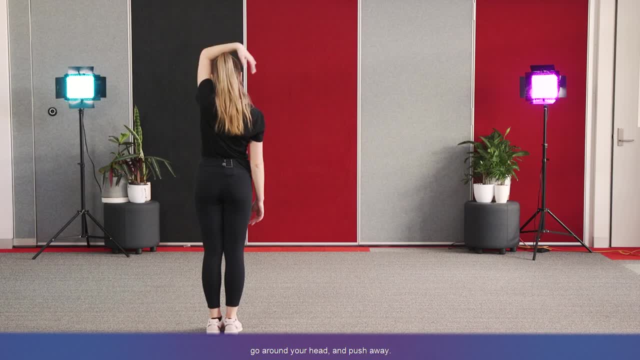 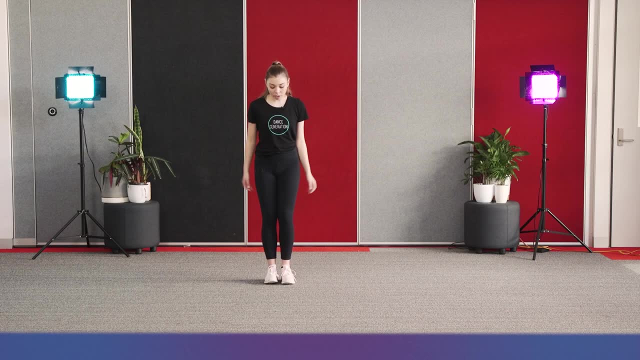 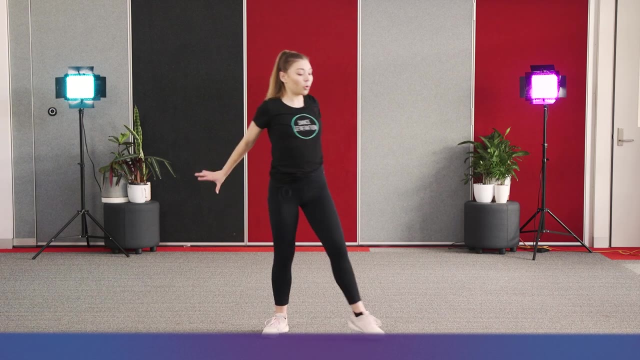 So we step up, you hold, goes around your head and push away. Let's try that from the start. Here we go, So we're looking down and then we look up, push through, push through, round together open rock. 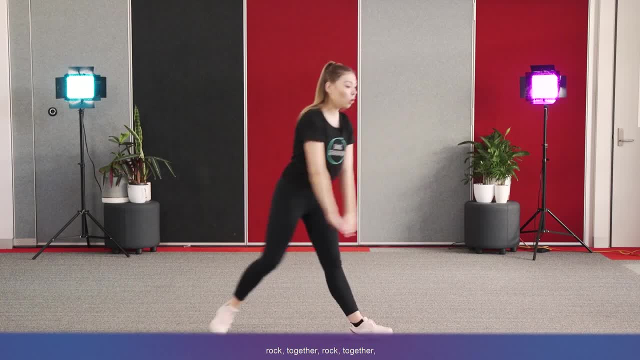 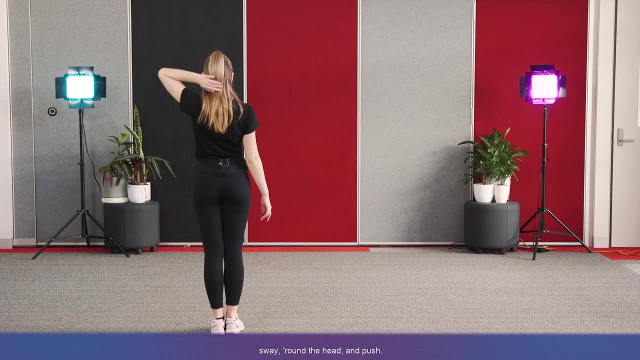 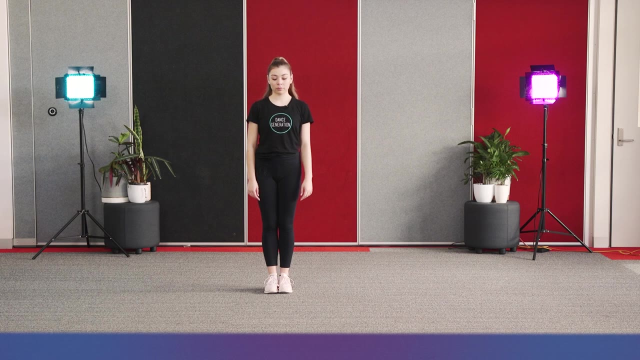 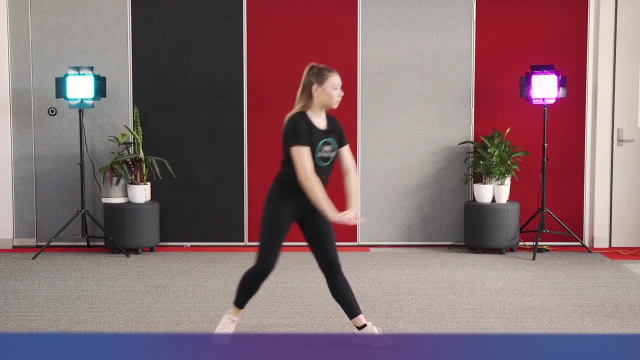 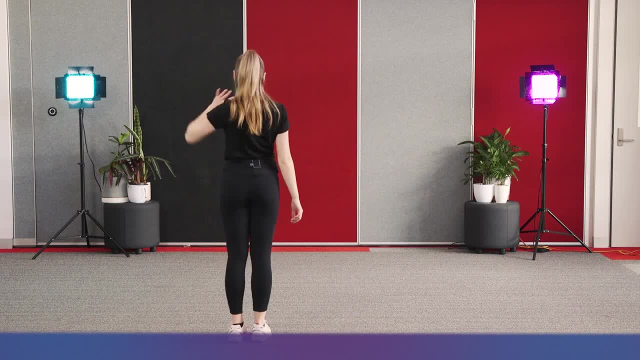 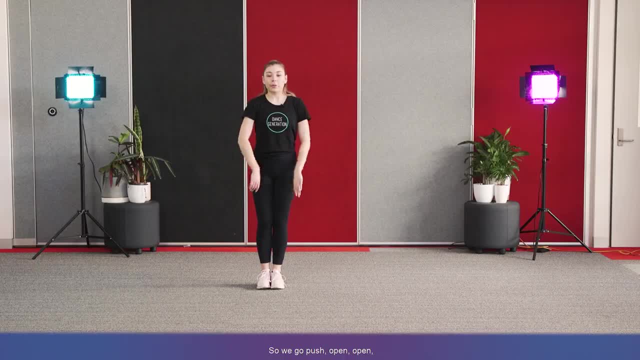 Oh my gosh, Let's try the other side. Good work, Let's quickly try out without music, and then we'll try it with music again. So we go, push, open, open round, PIIF, Push world, And we rock easy. 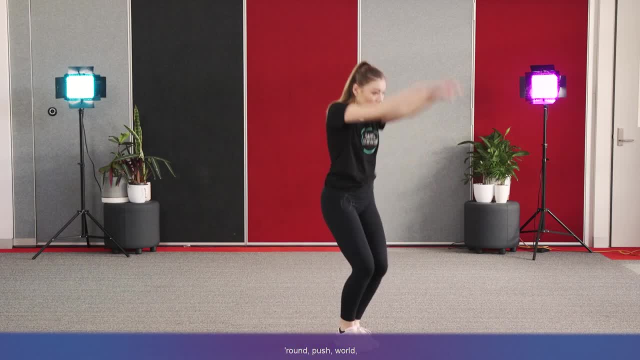 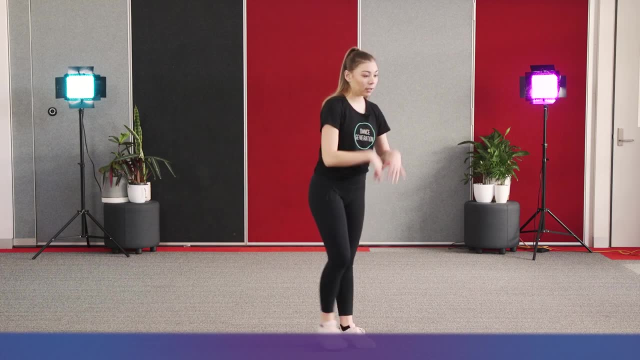 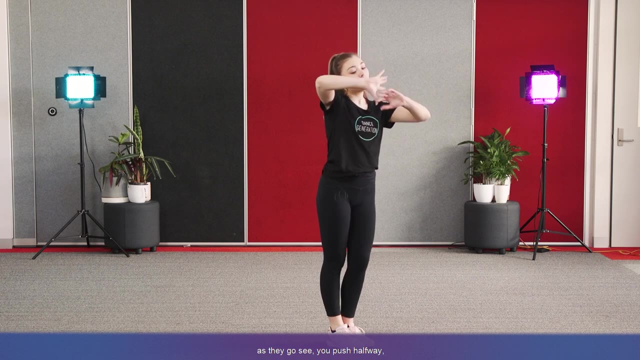 And we land across the girl Nice push whirl and we rock in rock, keep those hands down. so on the second rock they just come down as they go. C, you push halfway and then you extend, so that body is quite. 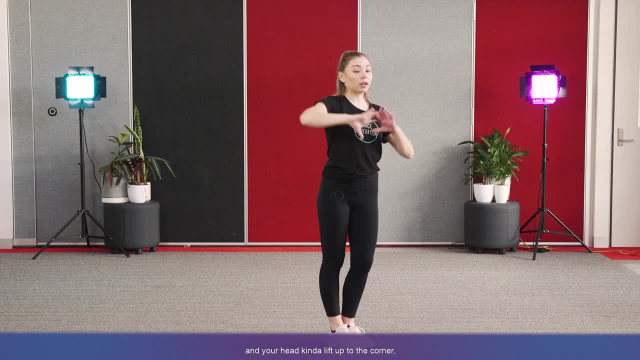 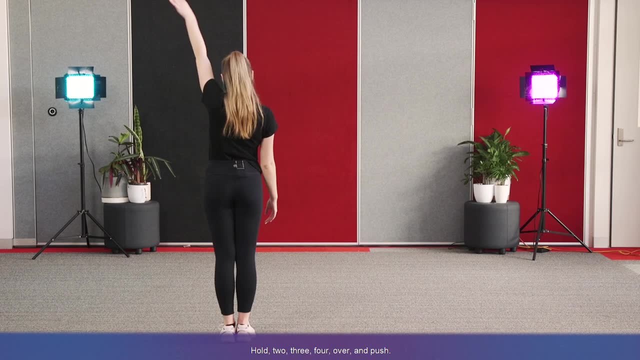 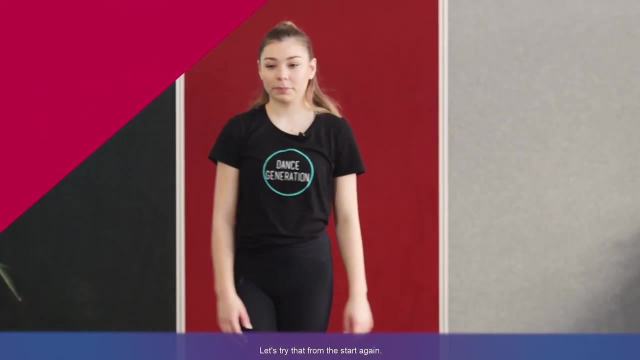 short and then it becomes longer. your chest and your head kind of lift up to the corner, because you look to the front and then you stretch up to the corner, hold two, three, four over and push. let's try that from the start again. here we go. 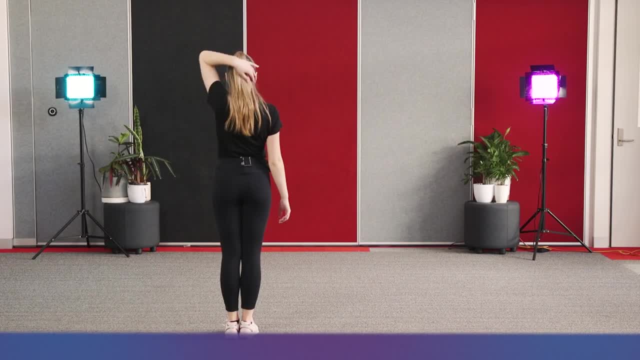 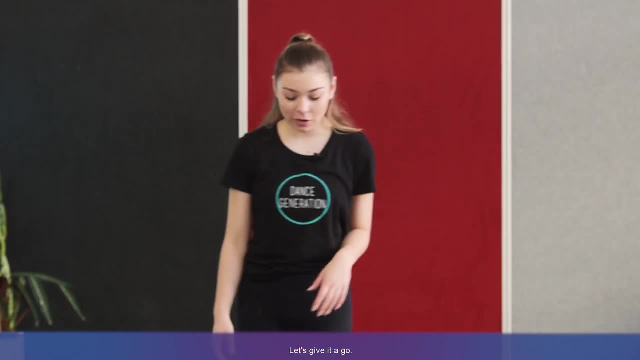 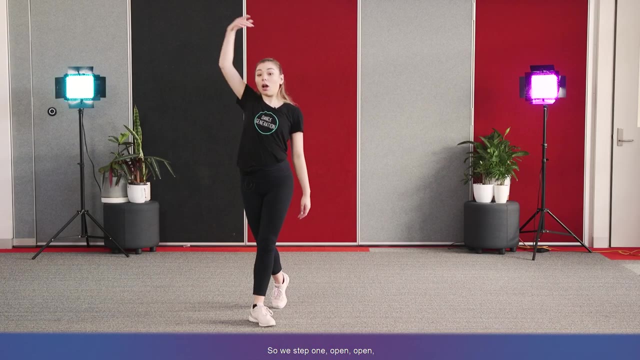 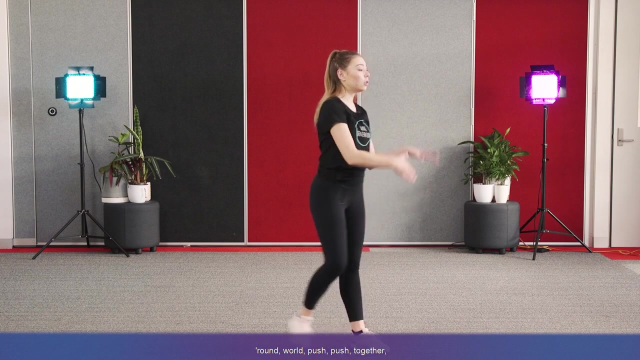 good work. so we're going to add on the next section. let's give it a go, we'll do it from the top and then we'll move on. so we step one open, open round, whirl, push, push. 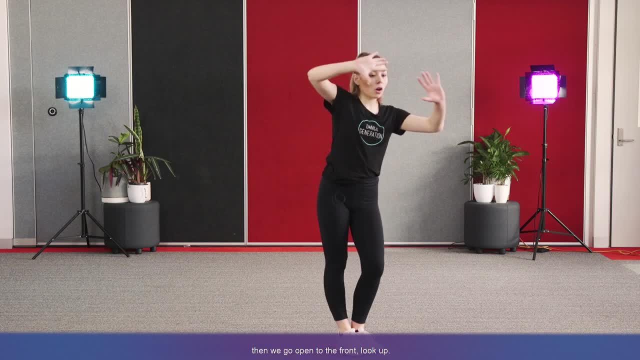 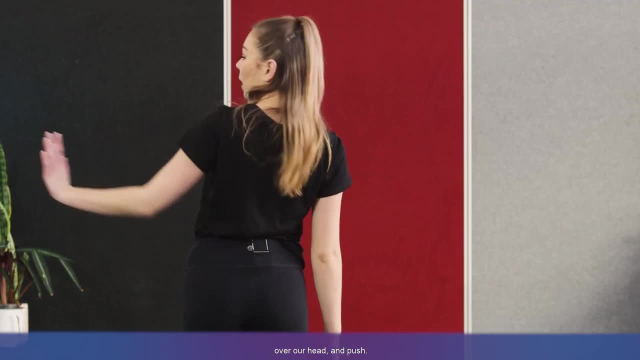 together. then we go open to the front. look up. it's kind of like a pause at the end. then we come up one, two over our head and push good. from there we walk to this shoulder, this. 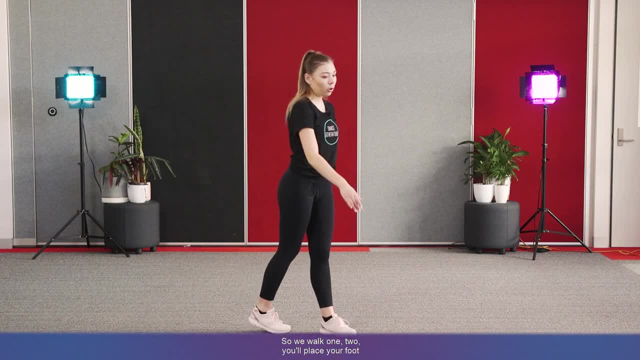 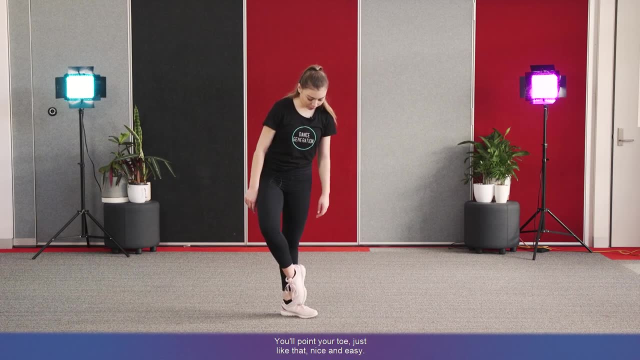 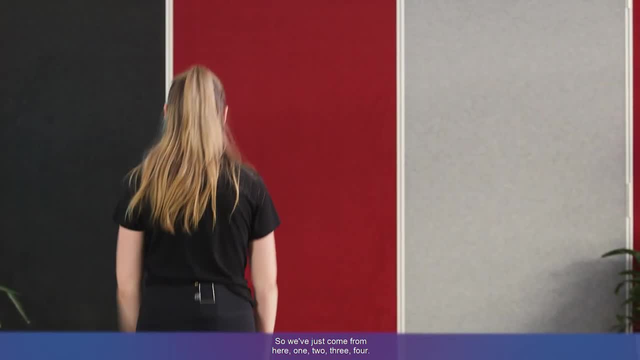 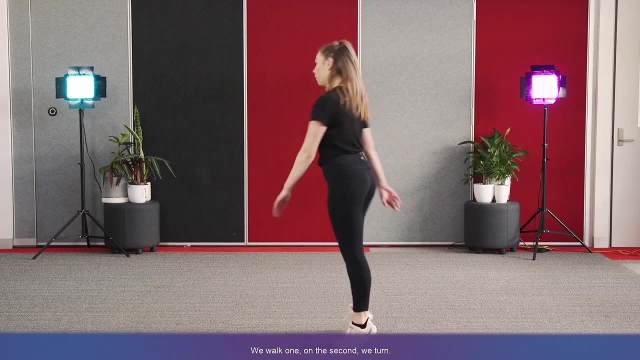 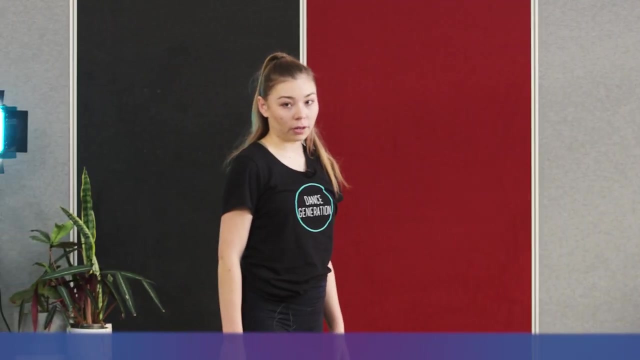 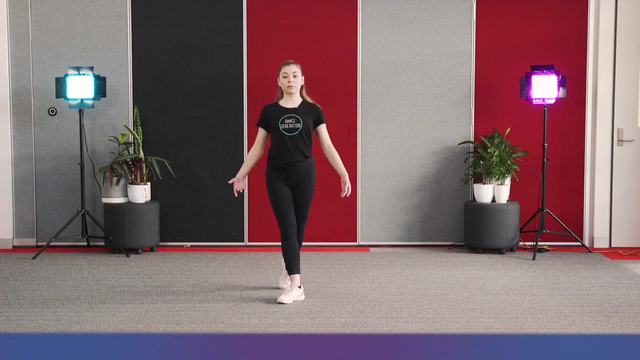 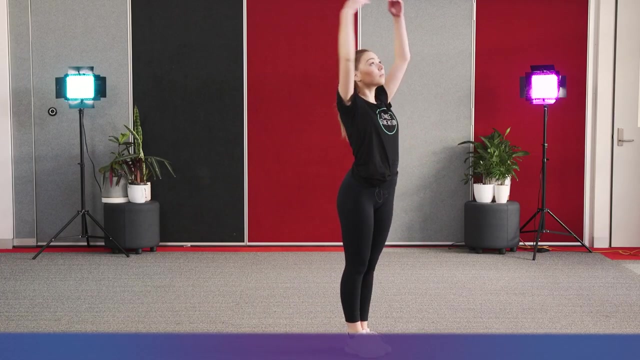 75,, 68,, 67,, 77,, 78,, 78,, 58,, 79,, 89, one. on the second, we turn, step forward, back back, jump forward. yep, let's do that from the start. two drifters off to see the world. there's such a lot of worlds. 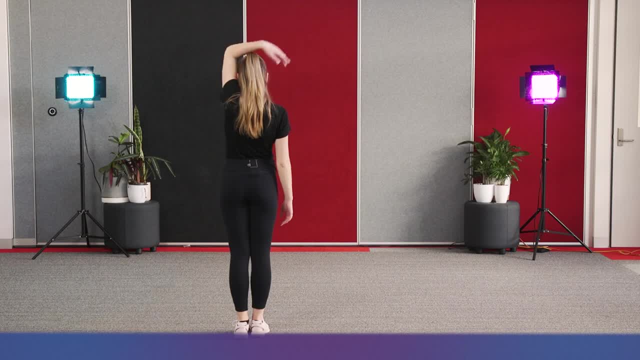 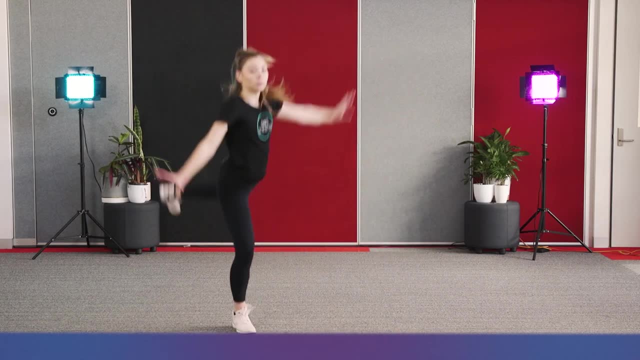 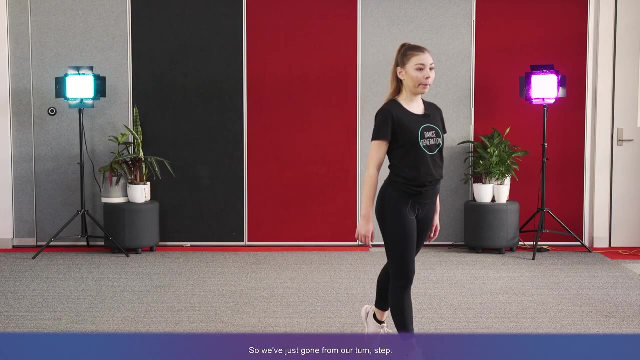 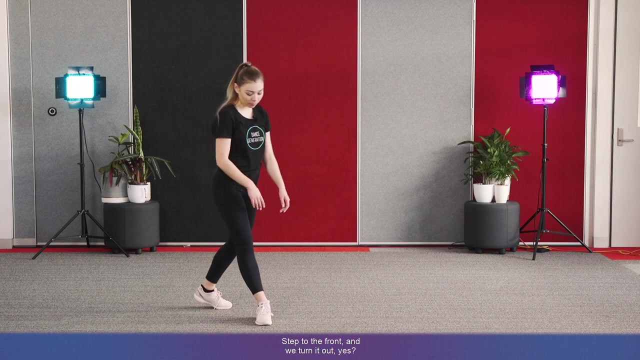 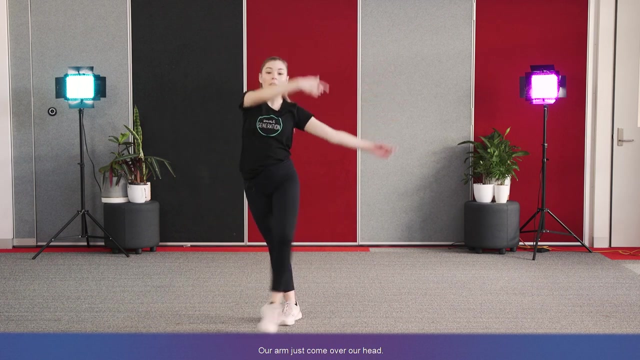 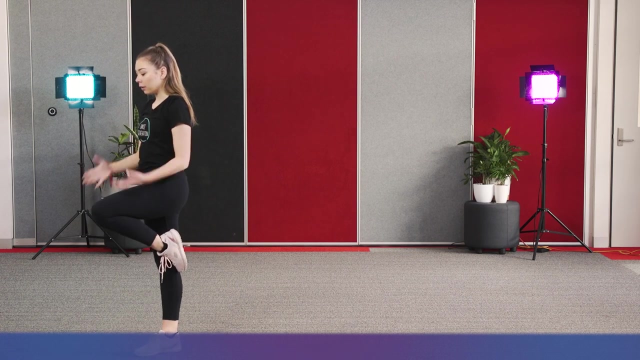 good work. so now we're going to add on. so we've just gone from our turn. step, step, step up rain bow. then we step towards the front, now step to the front, and we turn it out. yes, now i'm just come over our head. we step, step overhead in. yes, don't crunch your body. 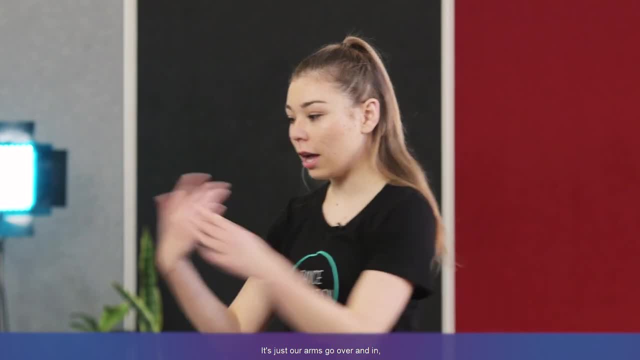 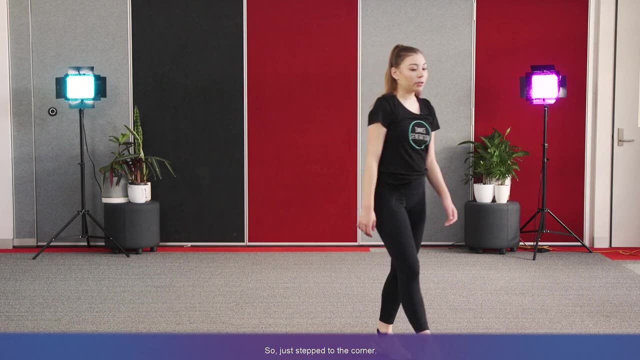 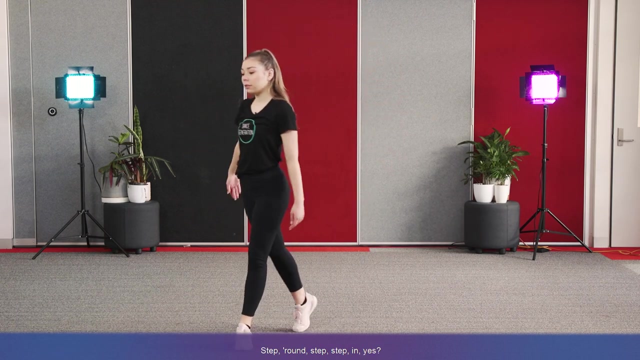 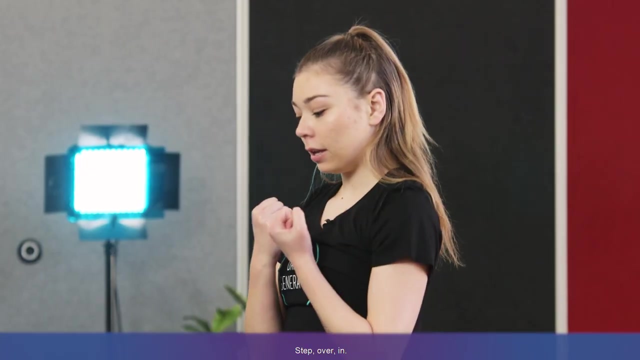 in. we want to keep it up, nice and tall- it's just our arms going over and in- and keep that knee nice and high. so we've just stepped to the corner. step, step, rain bow, step round, step, step in. yes, step over in. good, we'll try that. 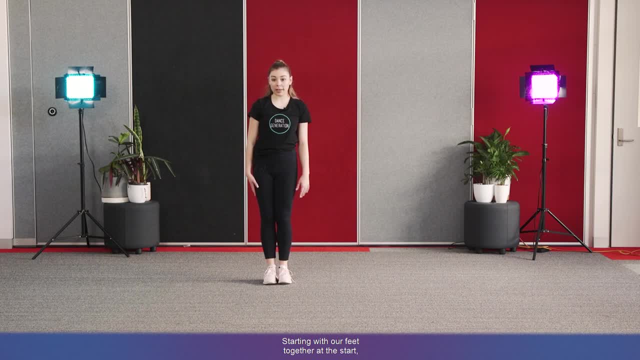 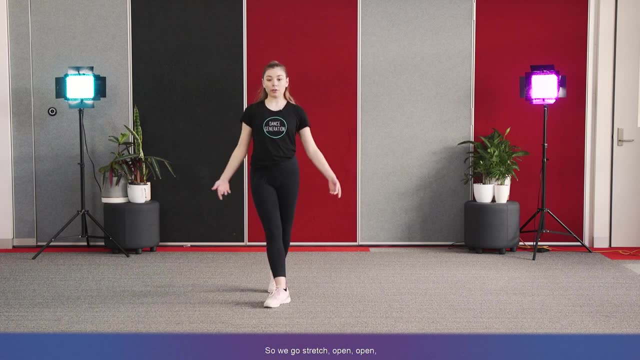 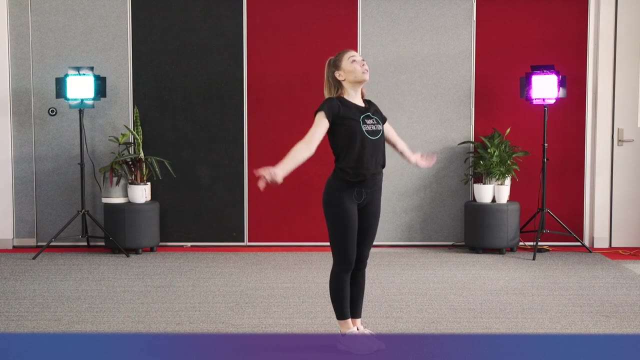 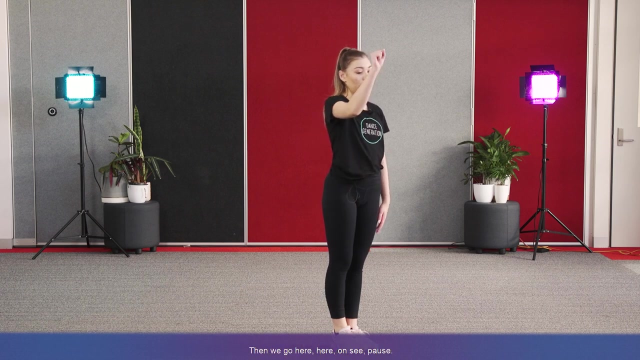 without music, and then we'll do it to music, starting with our feet together at the start, and I head down, and then, as soon as you hear that ding, you look up, so we go stretch open, open round, whirl, hold, sway and sway. very good, then we go here here on C pause. we're up one, two. 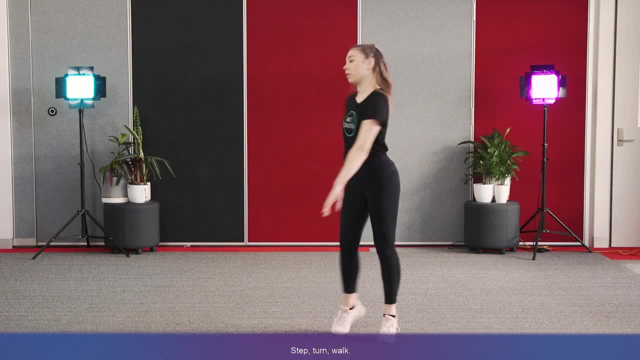 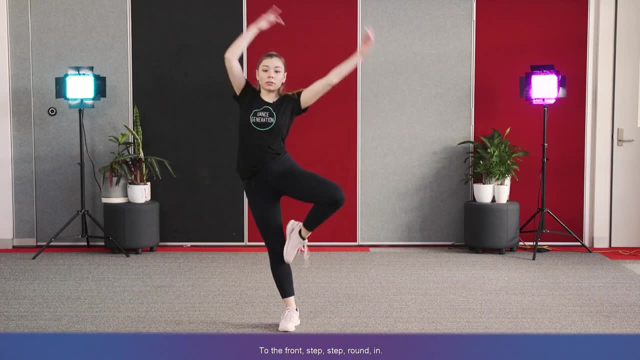 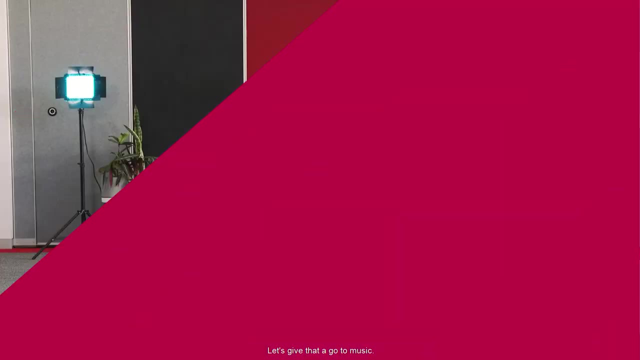 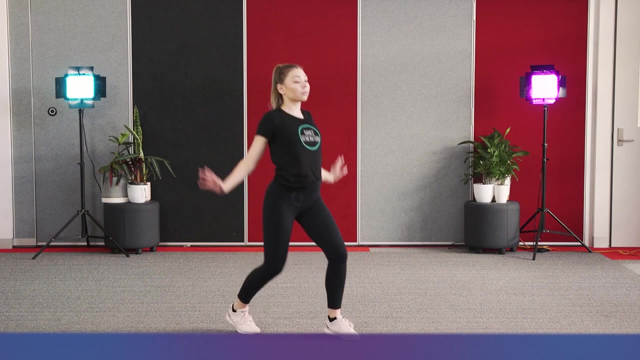 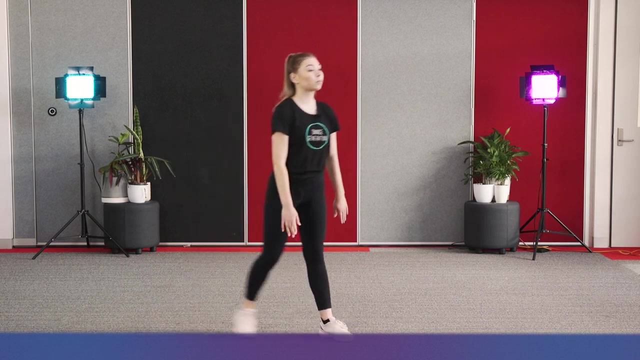 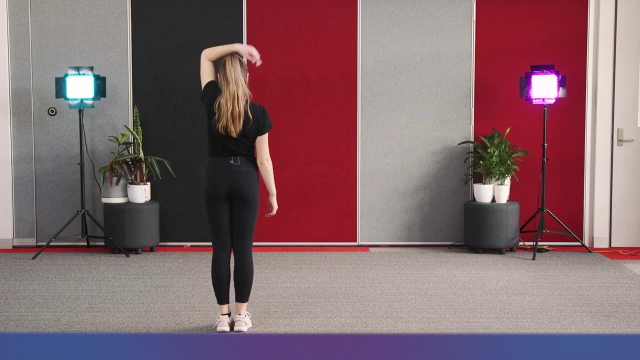 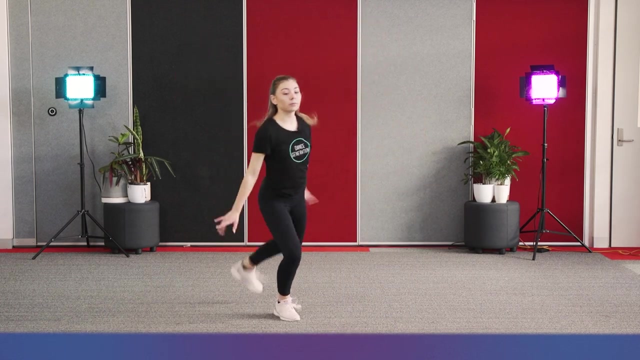 over three, four, step turn, walk, step, step up to the front, step, step round in. let's go give that a go to music. two drifters off to see the world. there's such a lot of worlds to see. we're after the same baby, baby, we're after the same thing. 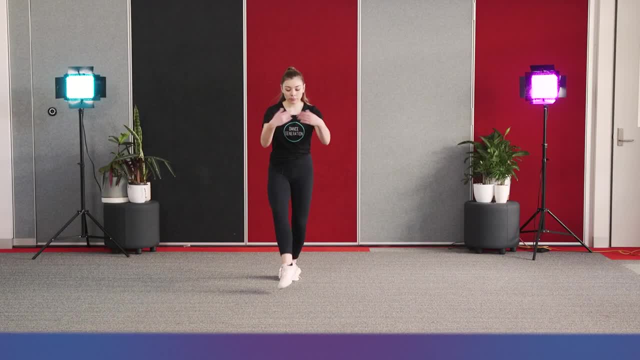 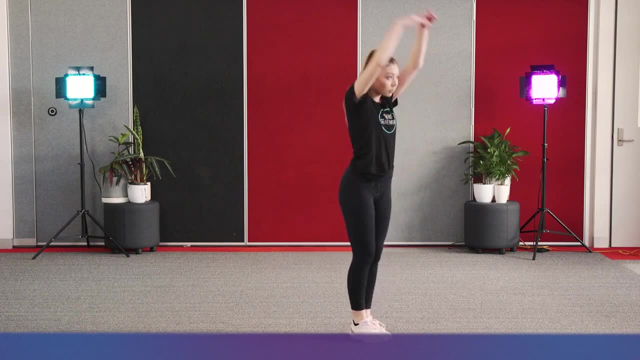 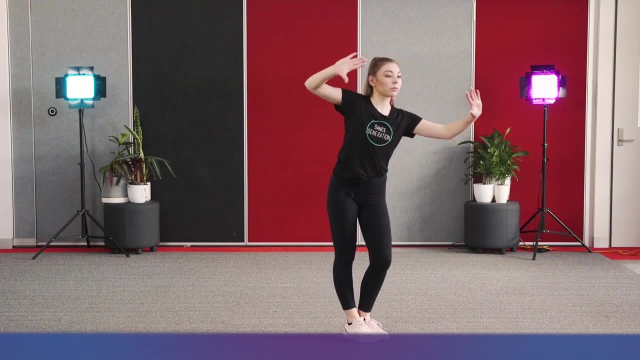 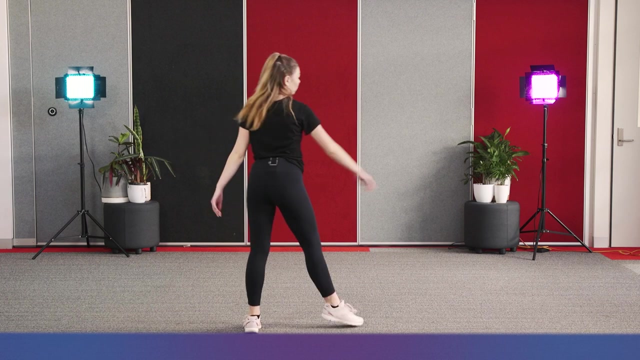 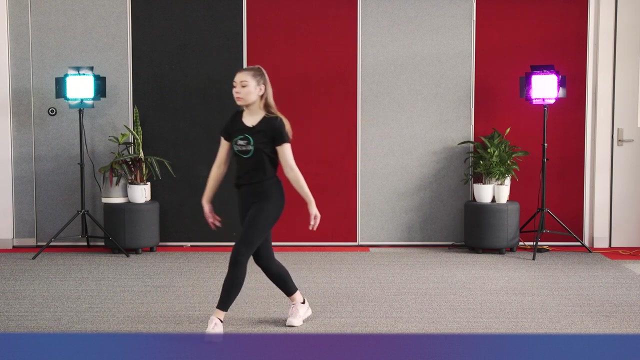 let's try that one more time to music, and then we can add on two drifters off to see the world. there's such a lot of worlds to see. We're after the same Rainbow's end, Waiting round the bend. Good, So now we're going to add on from here. 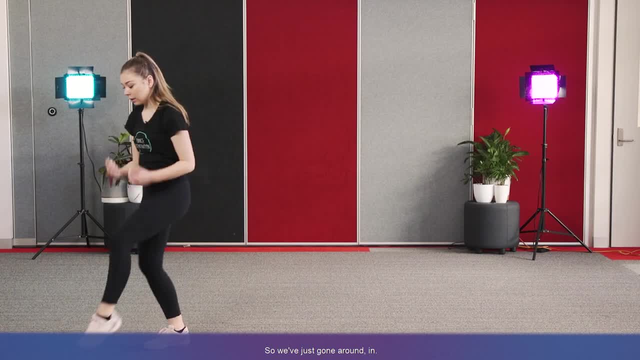 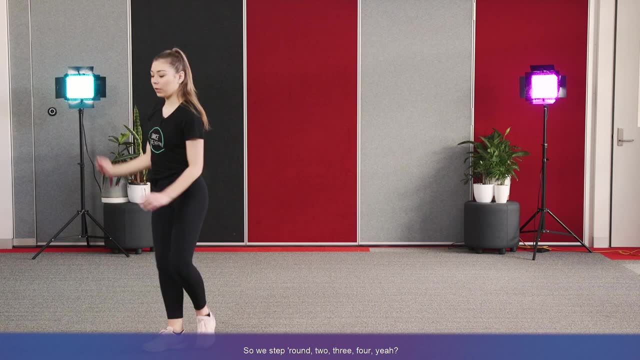 So I'm just going around in Step And as we step we're going to go in a circle. So we step round two, three, four, Yeah. so we're just going in Step. We step onto our right leg as we go around. 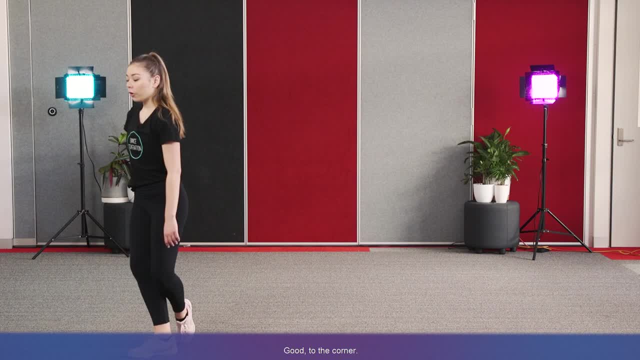 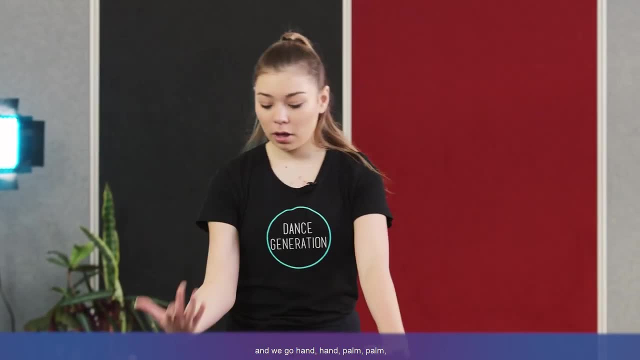 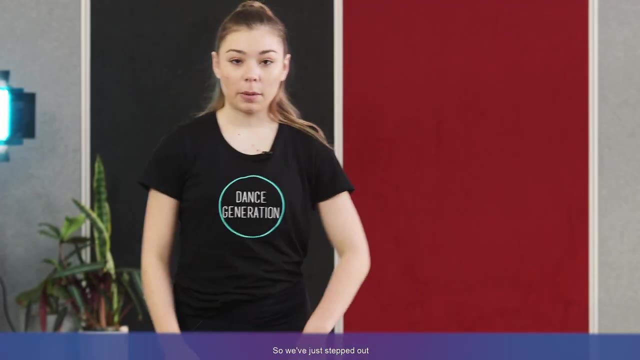 One, two, three, four, Good To the corner. Then we step to the front And we go hand hand, palm, palm Up up, head roll, Yep. So we've just stepped out after our little turn. 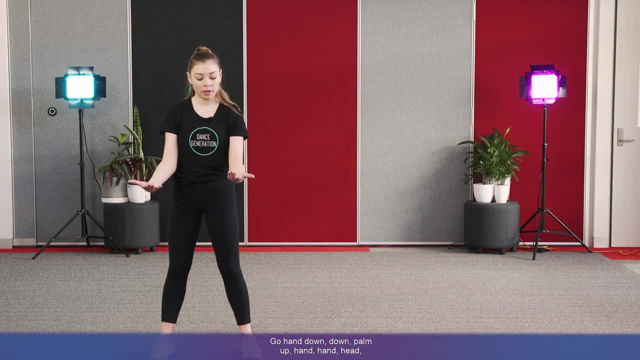 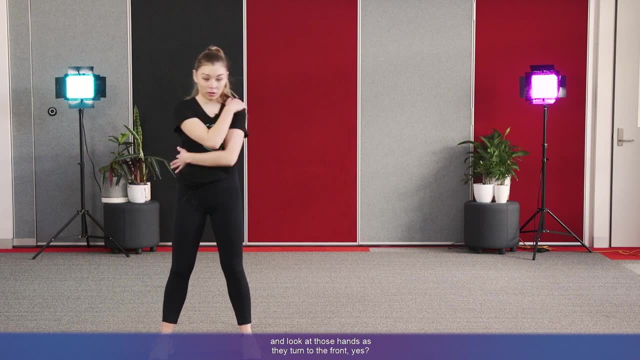 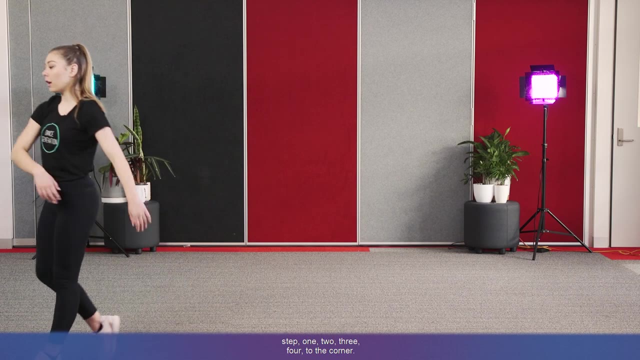 We go hand down down, palm up, hand, hand head And look at those hands as they turn to the front. Yes, So we've just gone step round in step one, two, three, four. 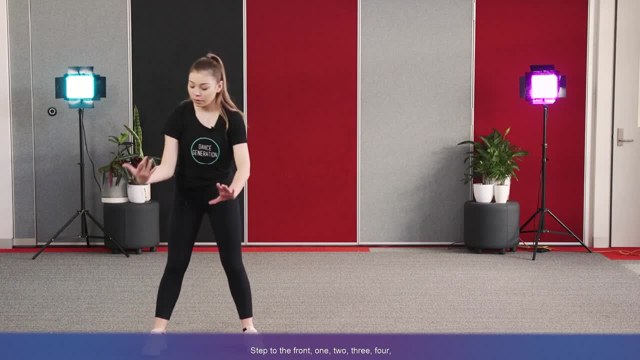 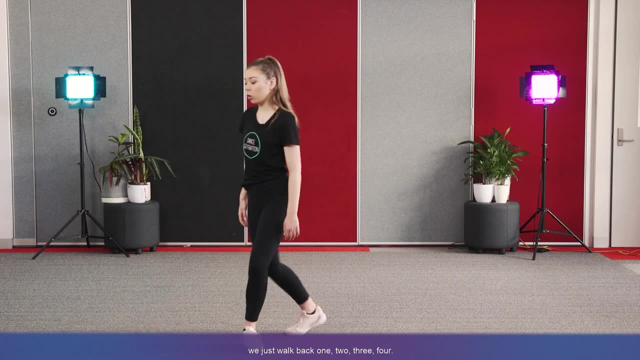 To the corner, Step to the front. One, two, three, four round round head, Yes, And then from here, Yes, Yes, And then from here we just walk back. one, two, three, four. 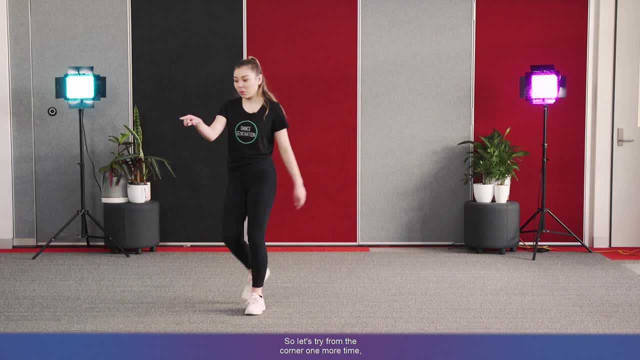 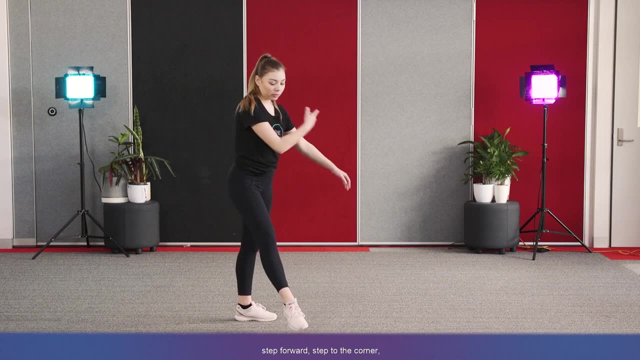 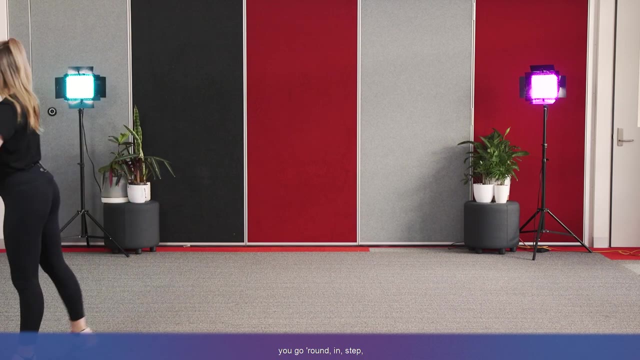 Almost like you're walking off stage. So let's try from the corner one more time and then we'll do it to music. So you've just done your good old rainbow: Step forward, step to the corner, You go round in step to your right foot. 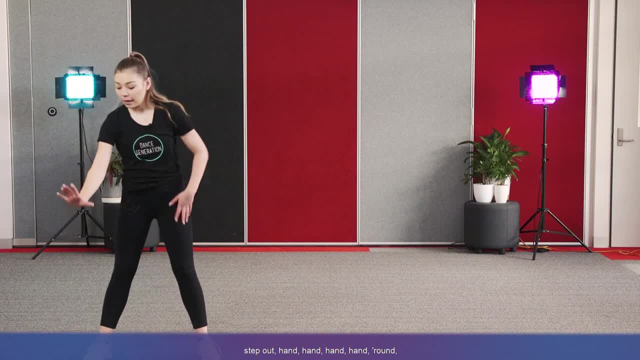 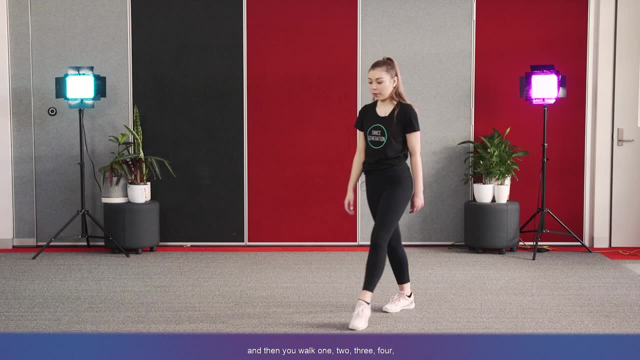 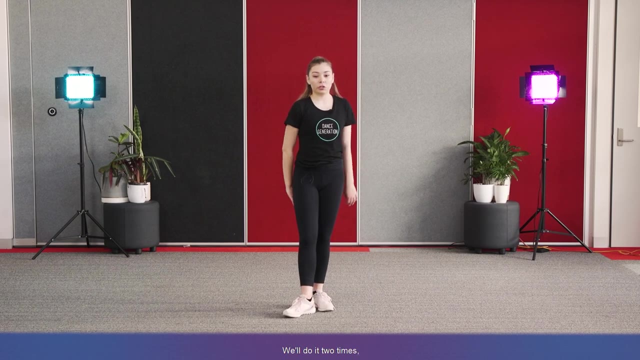 Two, three, four, Step out, Hand, hand, hand, And then you walk one, two, three, four, Almost back to the other corner, instead of walking straight on. Yes, Let's try that to music. We'll do it two times and then that is all. 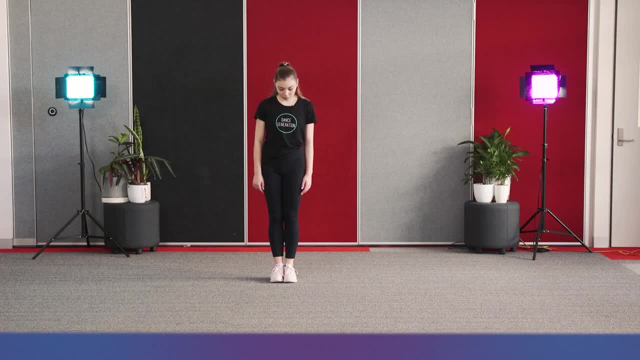 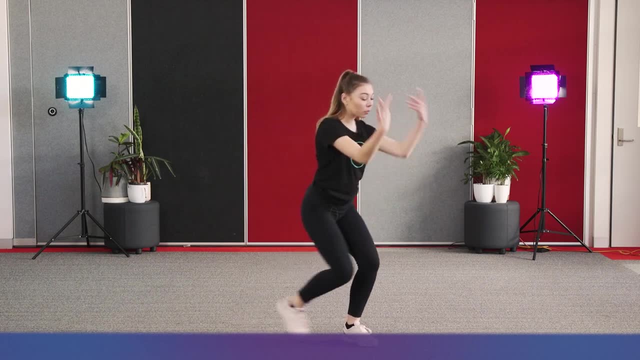 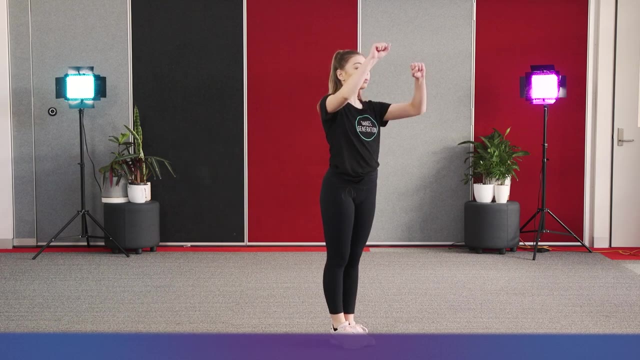 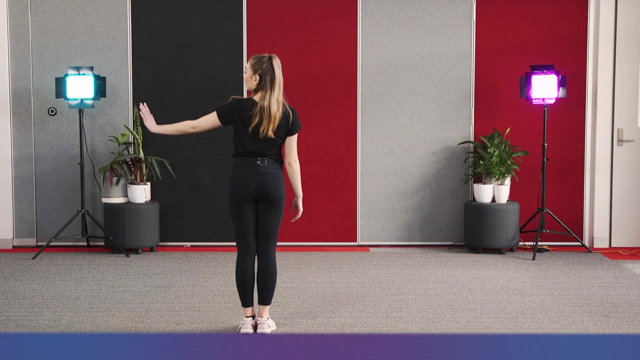 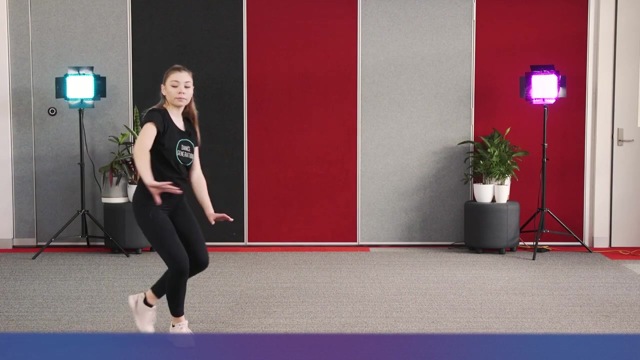 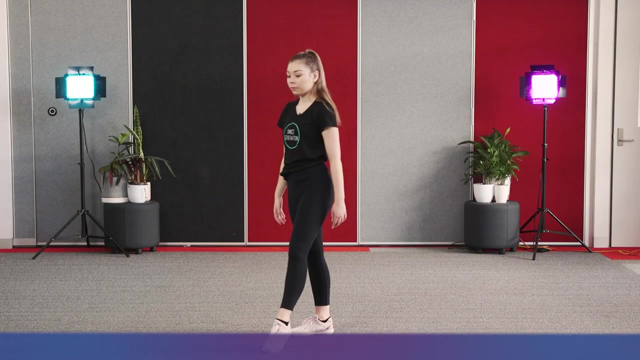 Go in your way to drifters Off to see the world. There's such a There's such a lot of worlds to see. We're after the same rainbow's end, wading round the bend, My huckleberry friend, Oh river. 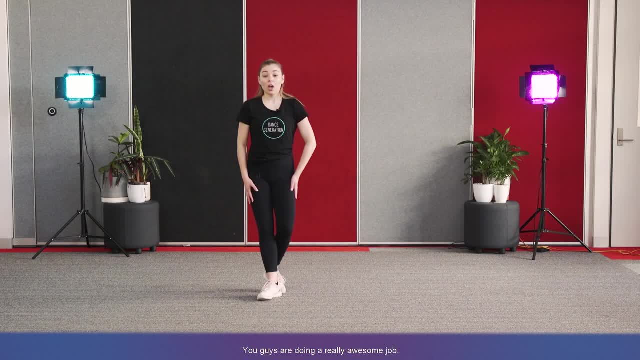 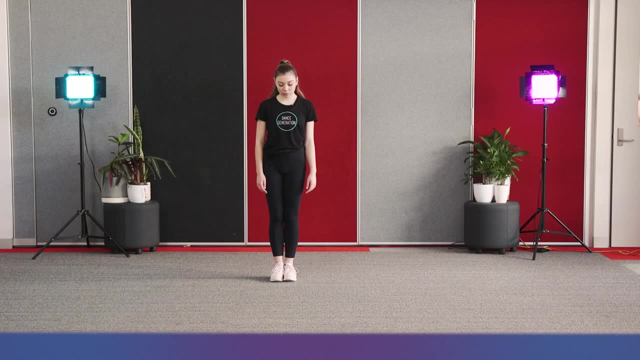 Good work. Let's try it one more time. You guys are doing a really awesome job. It's a little bit challenging, but it's a lot of fun, so just really feel the music and have a good time. Go in your way to drifters. 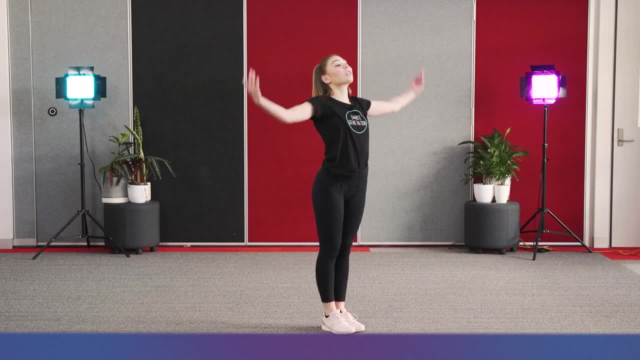 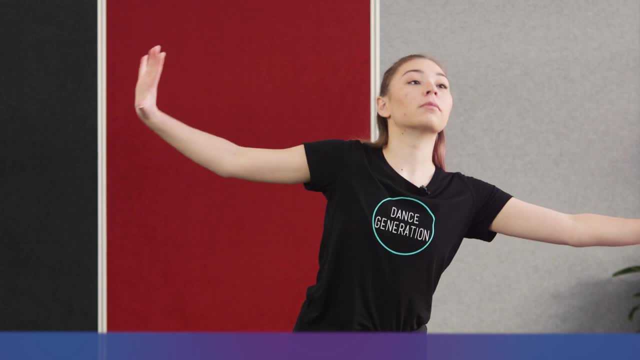 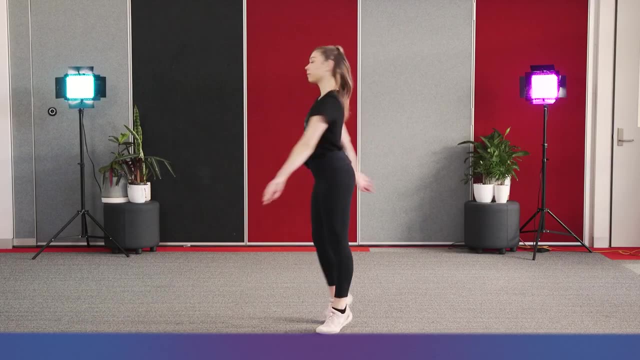 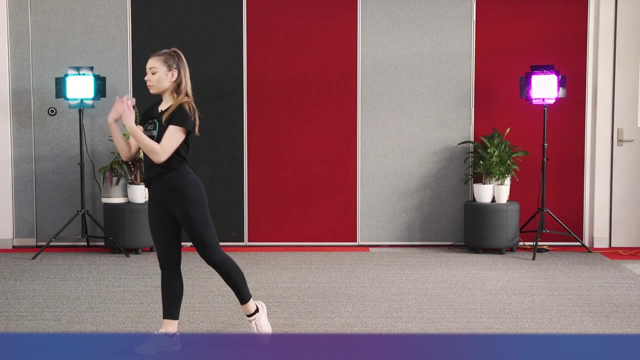 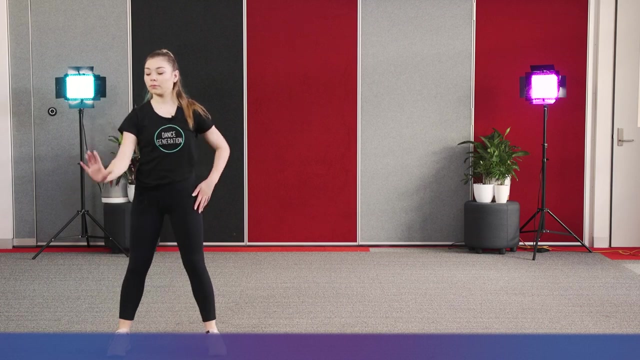 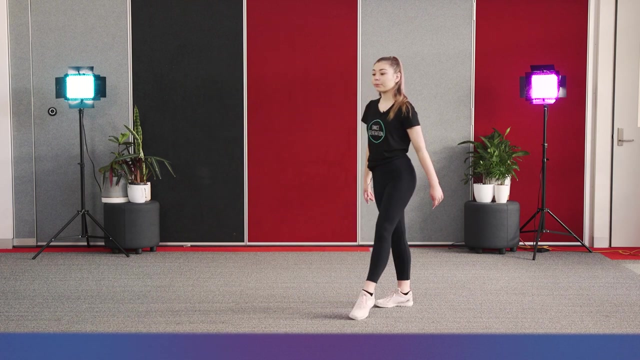 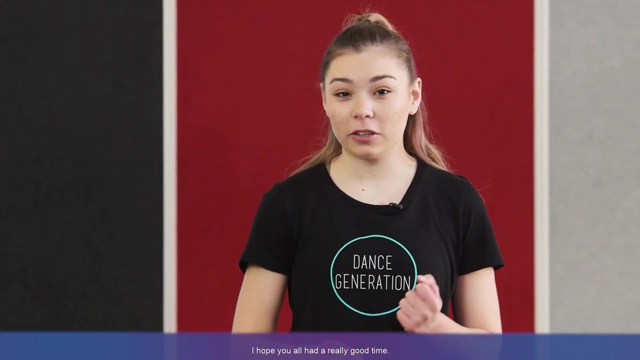 To see we're, after the same rainbow's end, Wading round the bend, my huckleberry friend, Moon river. Thank you guys so much for joining me in this class today. I hope you all had a really good time. You can follow us and join us at a dance class at Dance Generation. 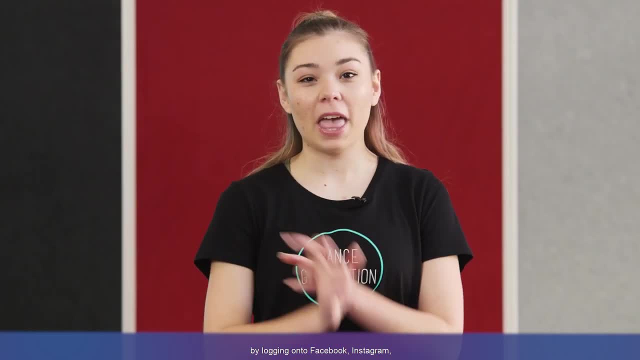 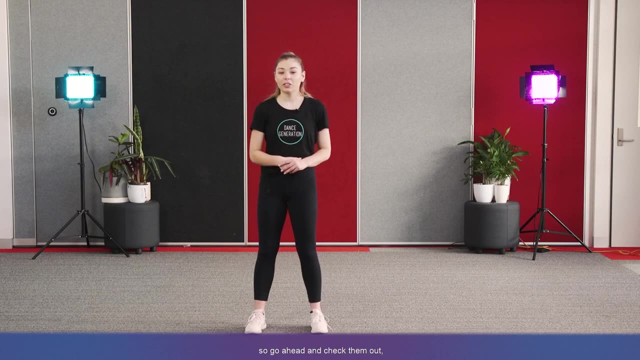 by logging on to Facebook, Instagram and checking out our timetables, as I do teach lyrical, contemporary jazz and musical theatre, So go ahead and check them out and I might see you in the next class. See you in my next class, or two.